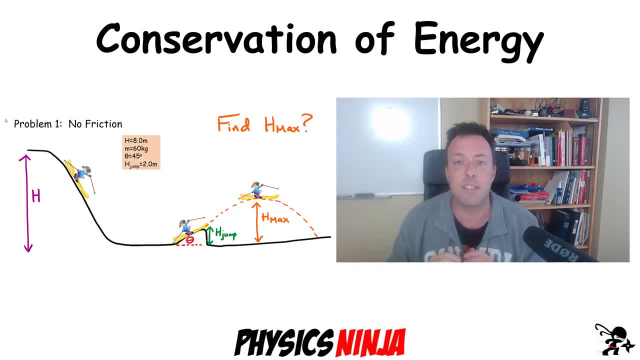 my goal is to calculate what is the maximum height of this skier. Now, in the second problem, what I'm going to do is I'm going to add a little bit of friction here down at the bottom of the hill in this kind of flat part. Okay, what that does now is: how do we introduce friction? 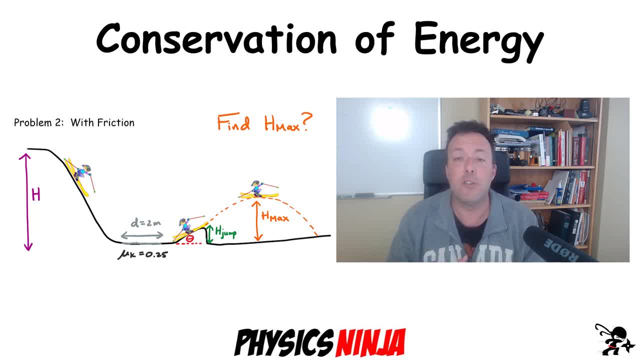 into energy problems like this. First, they're going to lose some mechanical energy and we're going to convert that to heat because there is work done by the force of friction. So I want to show you how you would modify the equations And again, at the end, my goal is to solve what is. 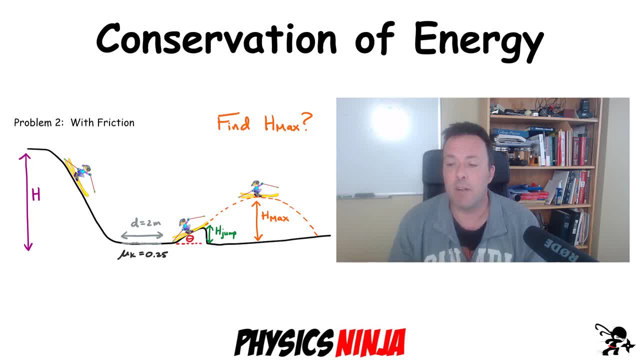 the maximum height that this skier is going to attain. Now, clearly, in the second case, probably not going to go as high as the first case, right, All right. so, like with all my videos, if you like it, give it a thumbs up, Consider subscribing to my channel. It's the best way to support. 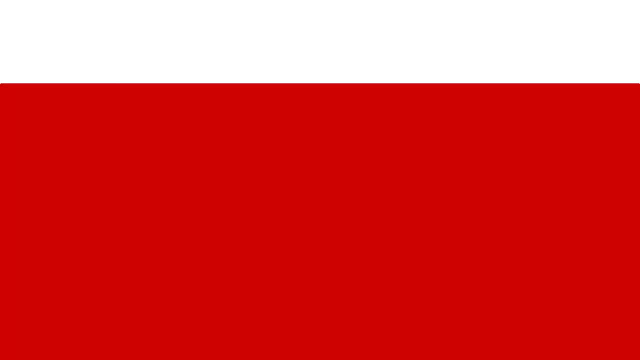 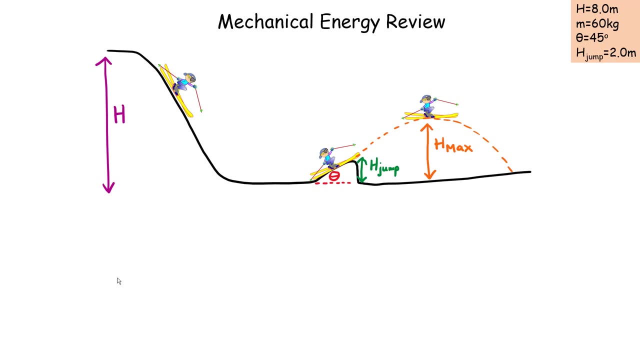 what I do. Okay, let's get started. All right, before kind of looking at this specific problem, let's just review a quick review of mechanical energy. Now, in this problem here, we have two forms of energy. All right, we're going to have kinetic energy. Kinetic energy is energy due to. 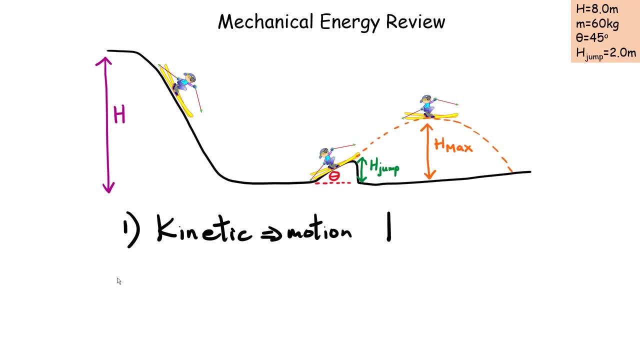 the motion of the skier, Okay. and kinetic energy. usually you write it with the letter K and the value is always the same: It's one half m, the mass of the object moving, in this case the mass of the skier, multiplied by the speed squared, Okay. 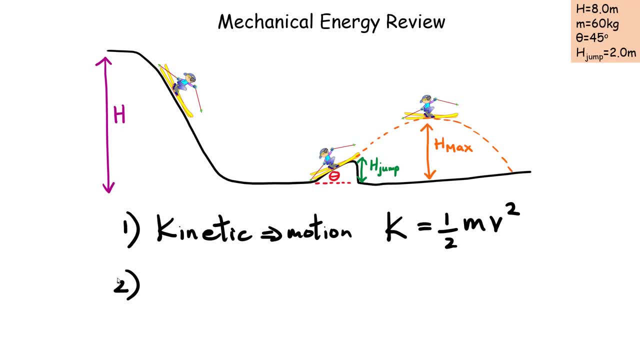 that's it Now. the other form of energy. what we're going to have here is potential energy. Okay, potential energy in this case is due to gravity, Okay, and usually we use the letter U for that case, and I'm going to write it as mg multiplied by y. Now there is something very 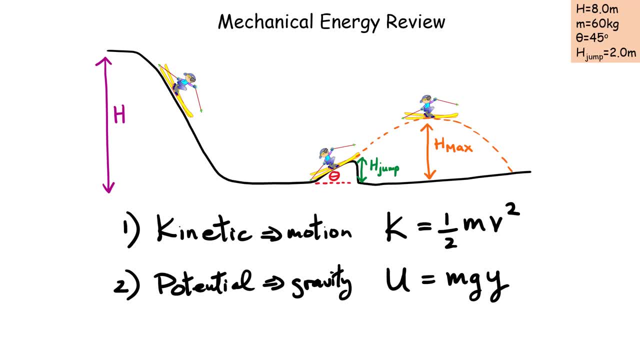 important here. We have to set a zero somewhere in this problem. So we're going to have to set a zero somewhere in this problem. You have to pick where is y going to be zero? Now, clearly, in most cases, you want to set the ground equal to zero and then every point above this here would be a. 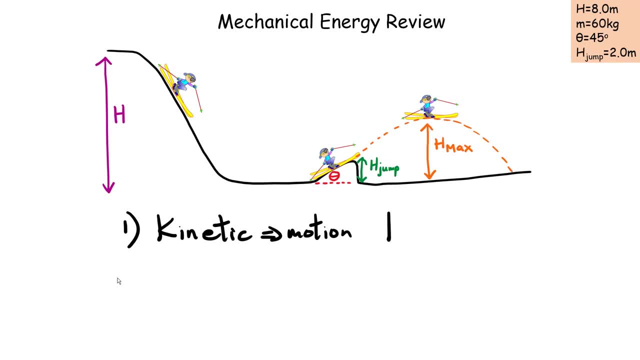 the motion of the skier, Okay, and kinetic energy. usually you write it with the letter K and the value is always the same: It's one half m mass of the object moving, in this case the mass of the skier, multiplied by the speed squared. 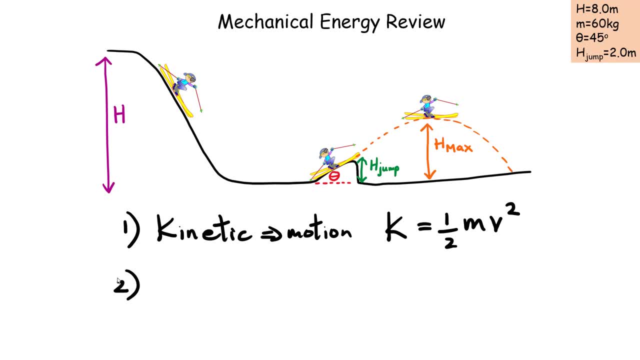 Okay, that's it Now. the other form of energy. what we're going to have here is potential energy. Okay, potential energy in this case is due to gravity, Okay, and usually we use the letter U for that case, and I'm going to write it as mg multiplied by y. Now there is something very 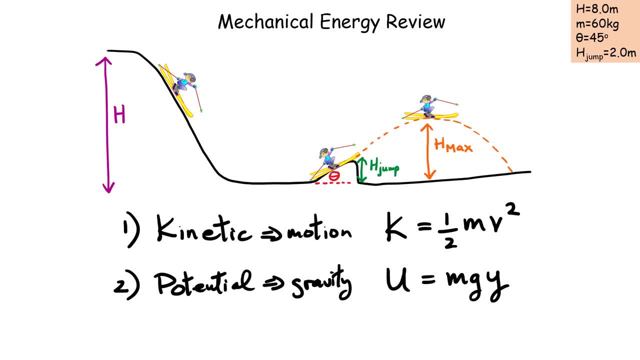 important here. We have to set a zero somewhere in this problem. So we're going to have to set a zero somewhere in this problem. So we're going to have to set a zero somewhere in this problem. You have to pick. where is y going to be zero? Now, clearly, in most cases, you want to set the. 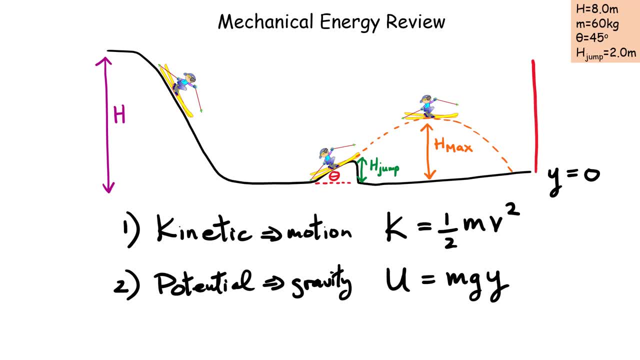 ground equal to zero and then every point above this here would be a positive y value. So that means that for this problem here my potential energy here at the ground would be equal to zero. Every value above that would have a positive value of gravitational potential energy. 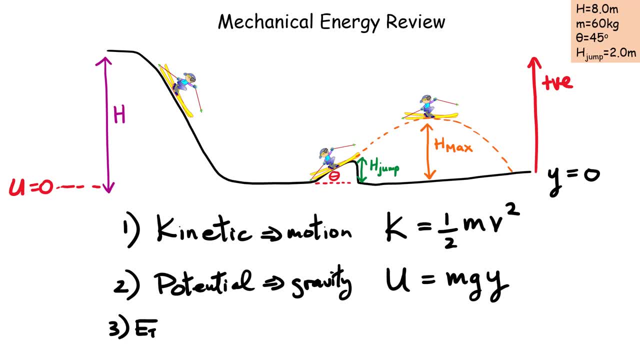 All right. and the last case? well, it's the total mechanical energy. Okay, total mechanical energy. So we're going to have to set a zero somewhere in this problem. You have to set a zero somewhere in this problem here, Okay, and then every point above this here would be a positive y. 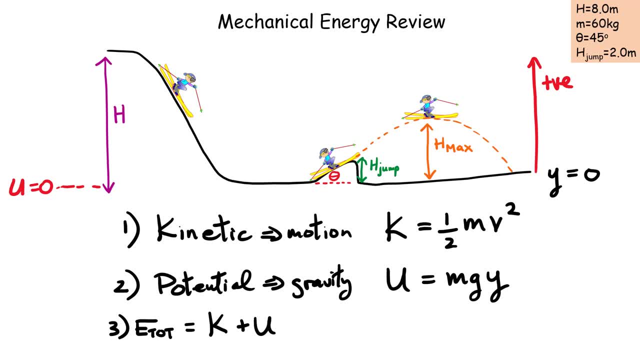 There's no continental potential energy here. Our internal mechanical energy is simply adding up the charge of graphite addition of per nim, which is equal to the total mechanical energy, colorfulosed herzlich, And that's it. So, if I write this in terms of the equations, here we have kinetic energy plus. 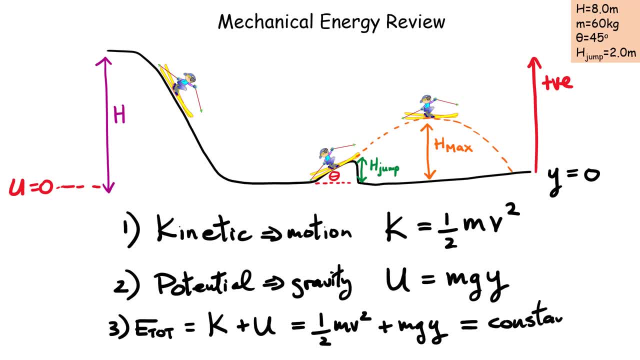 So in terms of the equations here, we have kinetic energy plus gravitational potential energy. Now, if there is no friction, this term here must be a constant value. It doesn't change. it simply means That the individual values of each of these energies can beсолv었어st hat, etc. I just wanted one way to 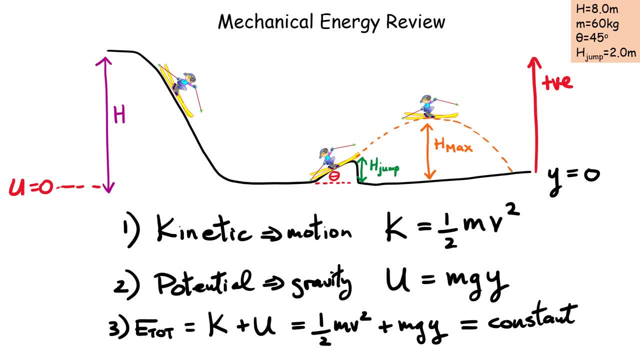 visualize a line chart and an example ofاد shrink, but you can obviously do it by changing your area here. these energies can change, And in my instance an change, But if I add them up together, they have to be a constant value. Okay, That is the statement. 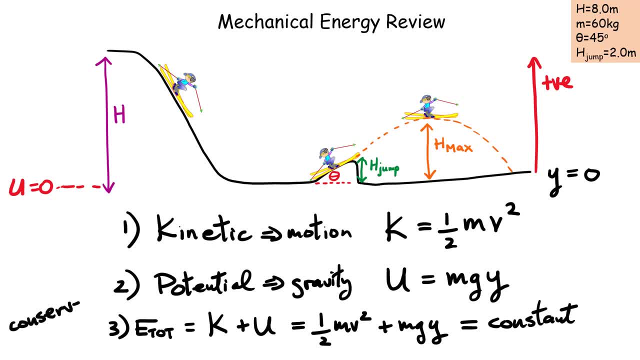 saying that energy is a conserved value. It does not change when the skier goes down, takes the jump and flies through the air in the absence of friction. All right, So let's go look at the first problem without friction and calculate this maximum height. All right, So we're going to look. 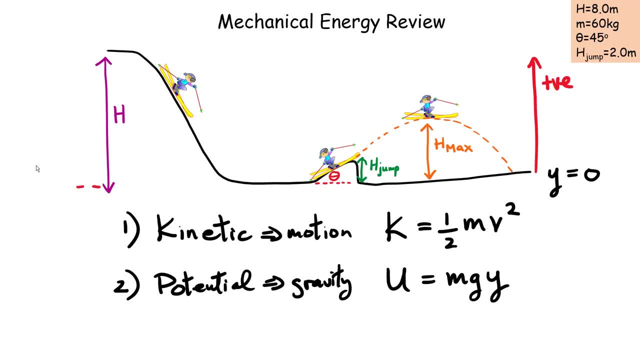 positive y value. So that means that for this problem here, my potential energy here at the ground would be equal to zero. Every value above that would have a positive value of gravitational potential energy. All right, and the last case? well, it's the total mechanical energy. Okay. 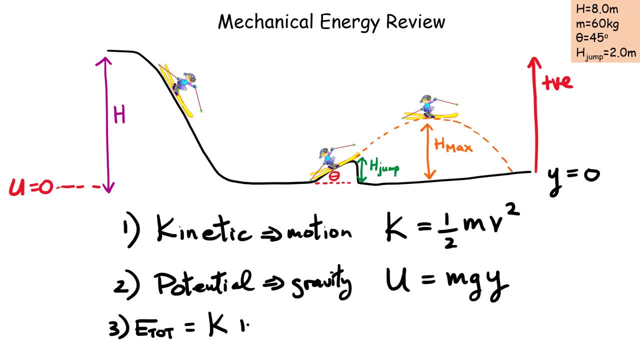 total mechanical energy. Okay, so we're going to have to set a zero somewhere in this problem. So the total mechanical energy is simply adding up the kinetic plus the gravitational potential energy at any point in this system. Okay, and that's it. So if I write this in terms of the 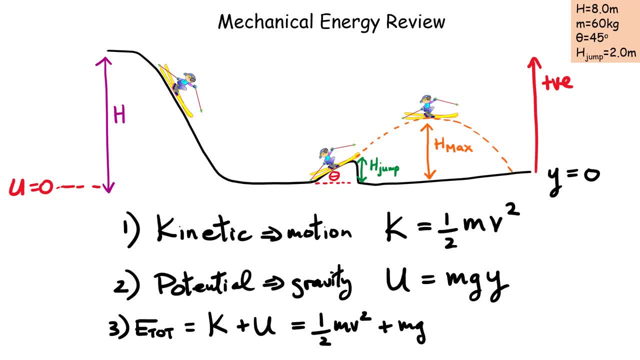 equations. here we have kinetic energy plus gravitational potential energy. Now, if there is no friction, this term here must be a constant value. It doesn't change. It simply means that the individual values of each of these energies can change. So if I write this in terms of the 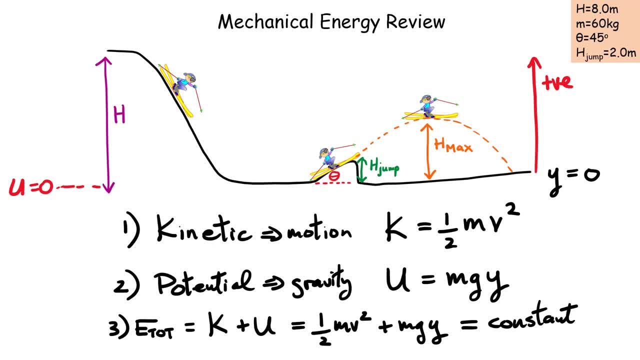 kinetic value of each of these energies. it doesn't change, But if I add them up together, they have to be a constant value. Okay, that is the statement saying that energy is a conserved value. It does not change. when the skier goes down, takes the jump and flies through the air. 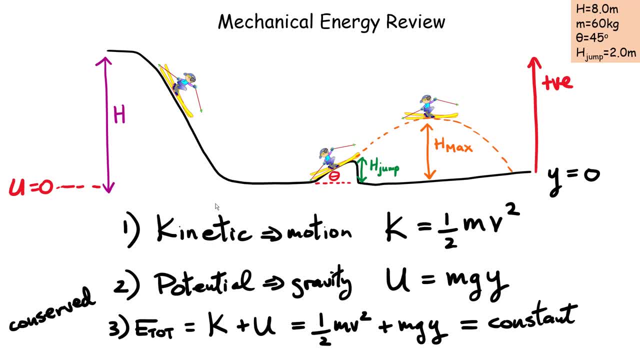 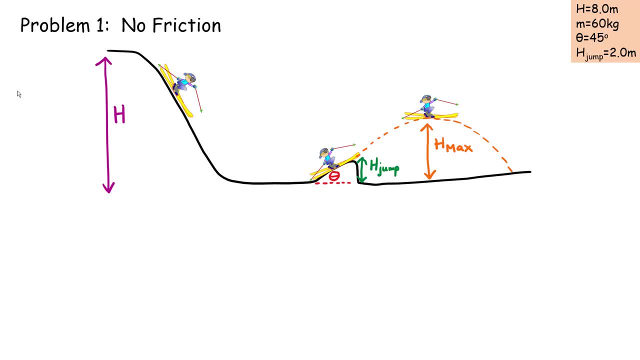 in the absence of friction. All right, so let's go look at the first problem without friction and calculate this maximum height. All right, so we're going to look at problem one. Here are the values that we're going to use: The height is eight meters, the mass is 60.. This angle of the jump. 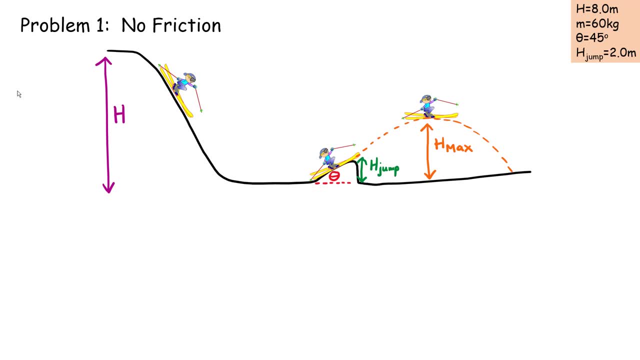 here is going to be 45 degrees, So we're going to look at this problem one. Here are the values that we're going to use. Let's just assume it's like a triangle here And the height of that jump is two meters. Okay, now to solve this problem again. the goal is to find H max, but we're going to do. 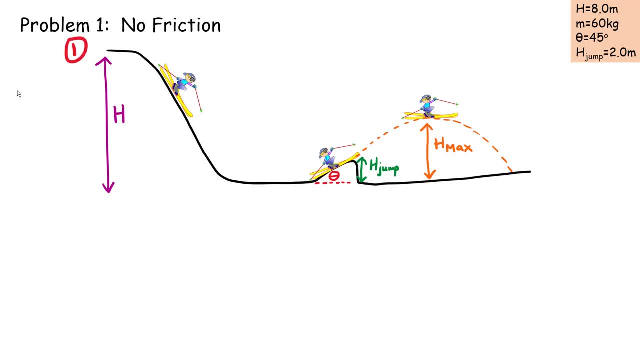 some intermediate steps here to highlight the method. We're going to look at three places. We're going to look at the top of the hill, We're going to look at the top of the jump right here. That's going to be number two, And number three is going to be at the top of the hill. Okay, 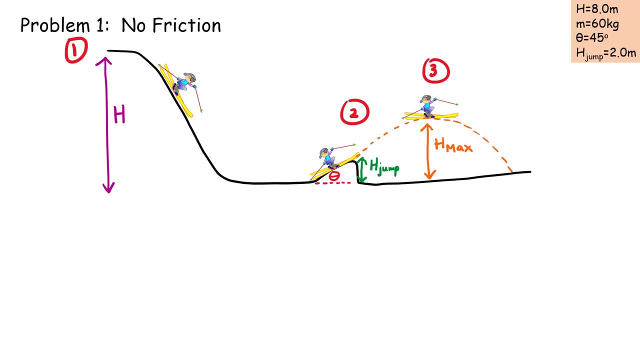 now what we want to do is set up our conservation of mechanical energy here for this system. So let's look at the total energy here at point one Again. the total energy would be the kinetic energy at the top plus the gravitational potential energy at the top. Now, in this case, 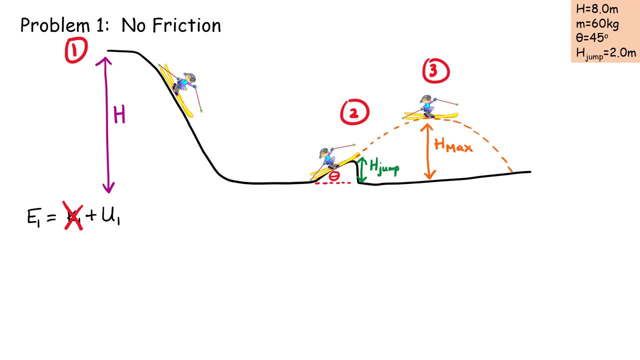 if I'm really starting at the top of the hill, I'm basically not moving. So there is no kinetic energy here. So all we have initially is gravitational potential energy. Now I can use the equation for gravitational potential energy, which is the mass times, little g times. 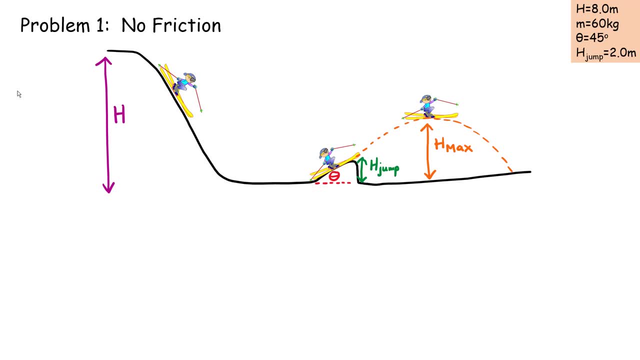 at problem one. Here are the values that we're going to use. The height is eight meters. The mass is 60. This angle of the jump here is going to be 45 degrees. Just assume it's like a triangle here And the height of that jump is two meters. Okay, Now to solve this problem again. the goal: 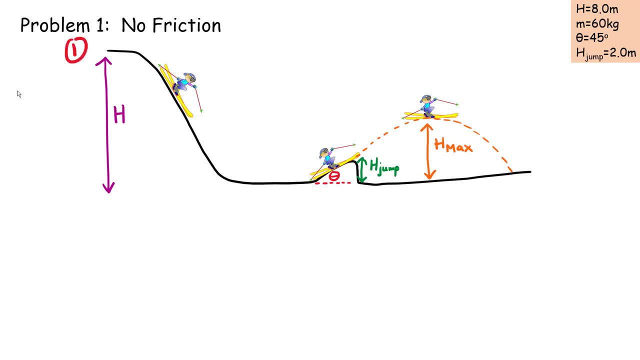 is to find H max. but we're going to do some intermediate steps here. to highlight the method, We're going to look at two, play, uh, three places. We're going to look at the top of the hill. We're going to look at the top of the jump right here. That's going to be number two. 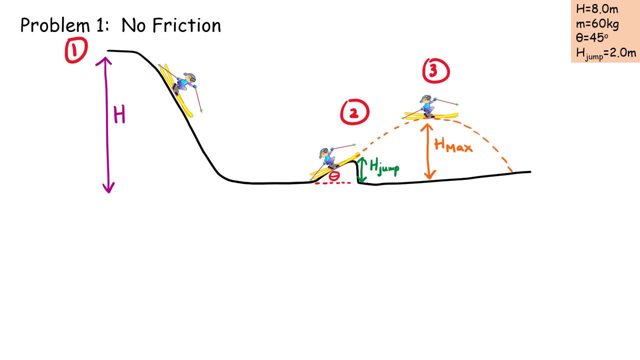 And number three is going to be at the top of the hill. Okay, Now what we want to do is set up our conservation of mechanics. We're going to look at the top of the hill, We're going to look at the energy here, uh, for this system. So let's look at the total energy here, at point one Again. 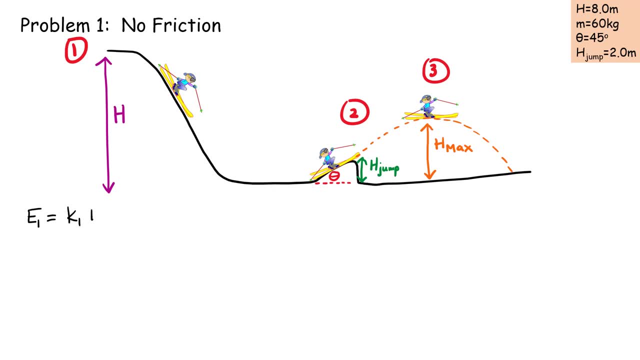 the total energy would be the kinetic energy at the top plus the gravitational potential energy at the top. Now, in this case, if I'm really starting at the top of the hill, I'm basically not moving. So there is no kinetic energy here. So all we have initially is gravitational potential. 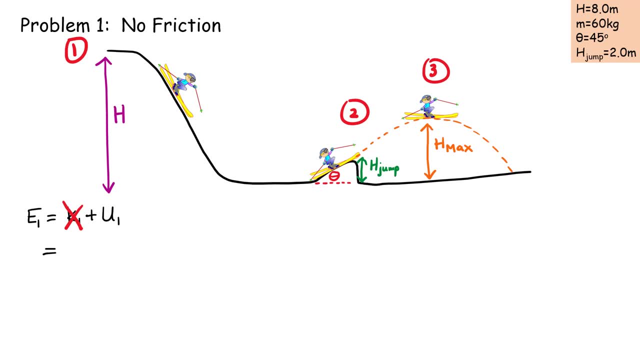 energy. Now I can use the equation for gravitational potential energy, which is the mass times little g times The height, in this case it's H. you could get a value for this. right, You could get a value If I just put 60,, uh 9.8, and then the height of that hill, 8.0,. I get a total energy in this case. 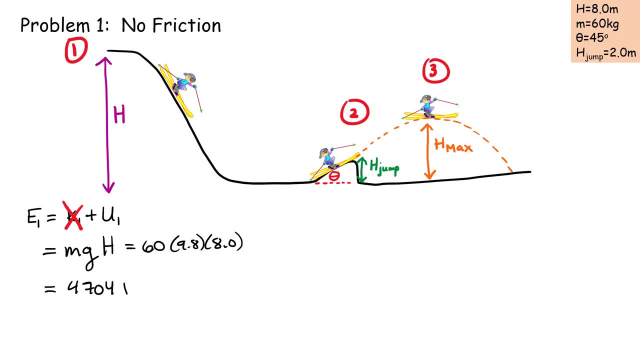 of 4,704.. And that's measured in joules. That's the total energy of the system. It doesn't change everywhere I go because there is no friction in this problem. Okay, Now let's look at the energy at the top of the ramp. Okay, At the top of the ramp, I'm going to look at the energy at the top of the ramp. 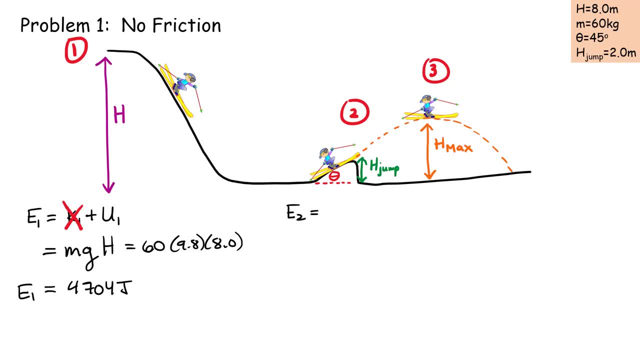 I'm going to call it E2.. E2 might have some kinetic energy because the skier is moving and he's above the ground, So he's also going to have some gravitational potential energy, All right. Well, the kinetic energy again, you can write as one half mv2 squared, Okay, Plus the potential energy. 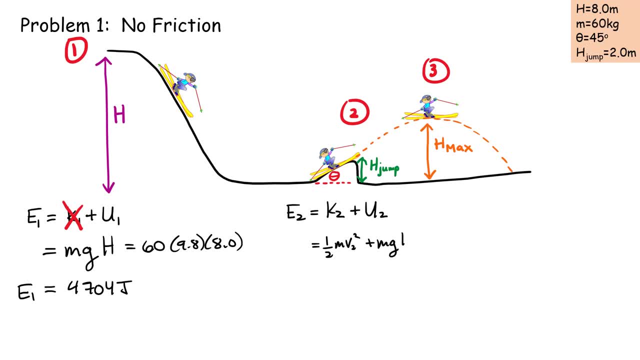 The potential energy is mg. What is the height over here? It's what's going to be the height of the jump. Okay, That is the total energy at 0.2.. Now, if you look at the different terms, you could calculate them. 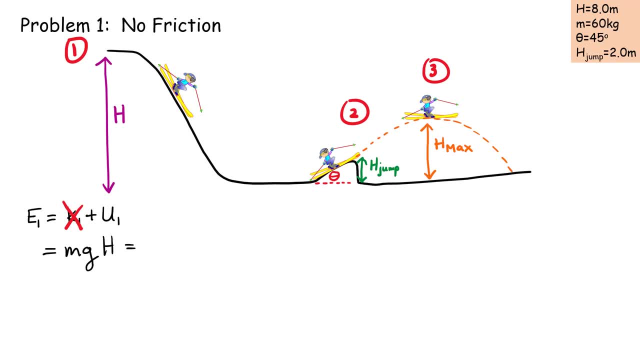 the height- In this case it's H. You could get a value for this right. You could get a value if I just put 60,, 9.8, and then the height of that hill, 8.0.. I get a total. 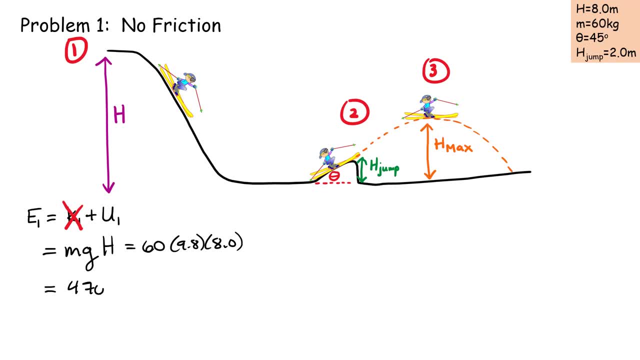 energy, in this case of 4,704, and that's measured in joules. That's the total energy of the system. It doesn't change everywhere I go, because there is no friction in this problem. Okay, now let's look at the energy at the top of the ramp. Okay, at the top of the ramp, I'm going to call it E2.. 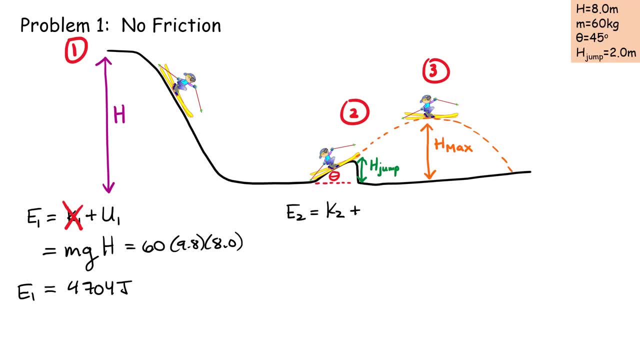 I'm going to call it the kinetic energy, because the skier is moving and he's above the ground, so he's also going to have some gravitational potential energy, All right. well, the kinetic energy. again, you can write as one half mv2 squared, okay, plus the potential energy, The 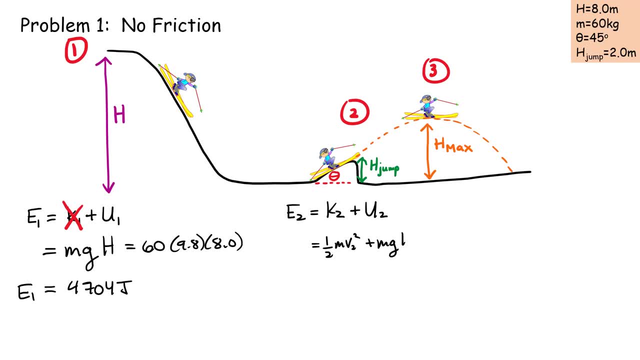 potential energy is mg. What is the height over here? It's what's going to be the height of the jump. Okay, that is the total energy at point two. Now, if you look at the top of the ramp, look at the different terms. you could calculate them individually, right, I could just first start. 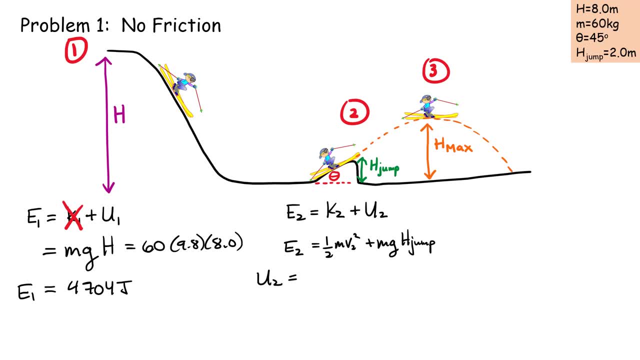 by calculating what is the potential energy over here, because that is just mg, the height of the jump. All right, substitute my values: I have 60. I have multiplied by 9.8, and then I have multiplied by h, jump is two meters. All right, my gravitational potential energy at the top. 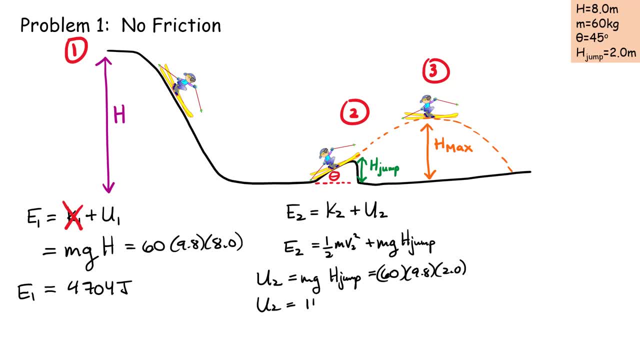 is much smaller than the original one. right, It's going to be 11, 176 joules. Okay, well, right away now. the only unknown now would be to find what is the kinetic energy now at the top right, The kinetic energy at the top. you can write it as well: what was? 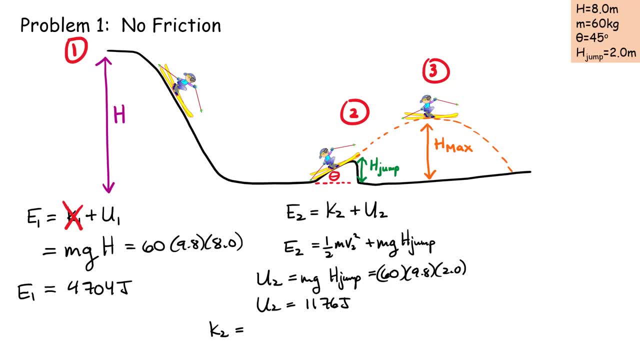 my initial energy, the total energy, e2.. Remember, e2 has to be equal to e1.. Energy is conserved everywhere in the system, so that means that the kinetic energy right here is simply this value, the gravitational potential energy at the top of this hill, So that here would be 4704,. 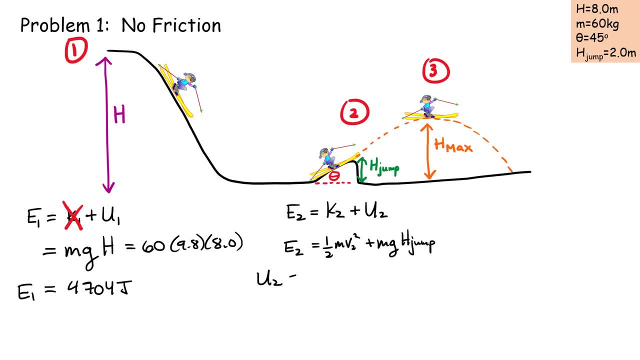 individually. right, I could just first start by calculating what is the potential energy over here, because that is just mg, the height of the jump. All right, Substitute my values. I have 60. I have multiplied by 9.8 and then I have multiplied by, each jump is two meters. All right, My gravitational 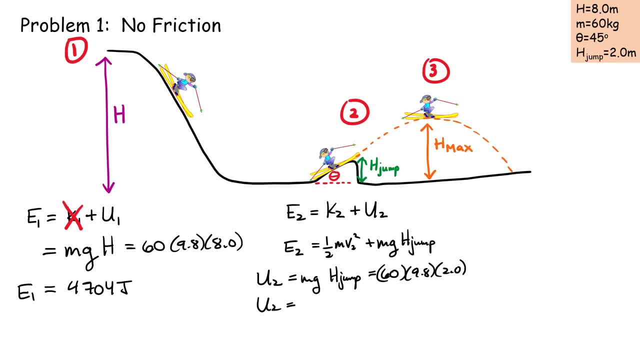 potential energy at the top of the ramp is mv2 squared. All right, So that's. the total energy at the top is much smaller than the original one. right, It's going to be 1176 joules. Okay, Well, right away now. the only unknown now would be to find what is the kinetic energy now. 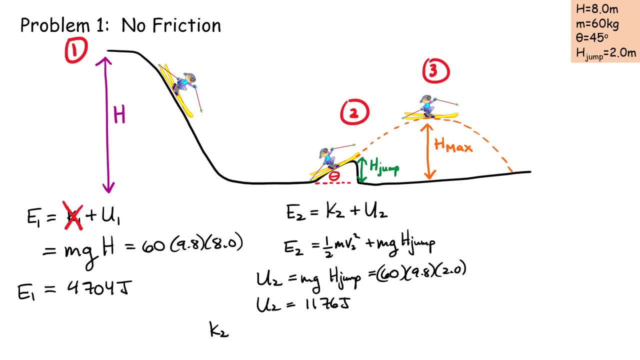 at the top right, The kinetic energy at the top. you can write it as well. what was my initial energy? The total energy, E2.. Remember, E2 has to be equal to E1.. Energy is conserved everywhere in 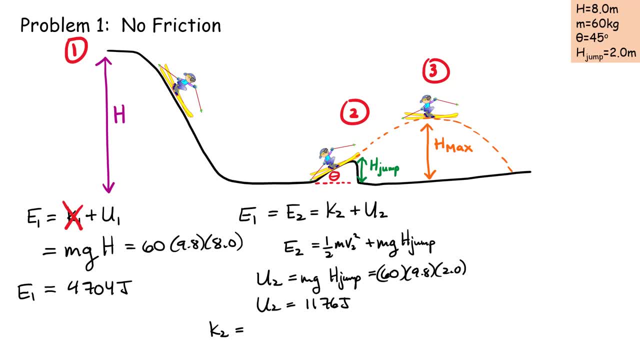 the system. So that means that the kinetic energy right here is 0.2 mv2 squared. All right, So that's simply this value, E1, minus the gravitational potential energy at the top of this hill, So that here would be 4704 and then minus 1176.. Okay, That gives me a kinetic energy of 3528 joules. 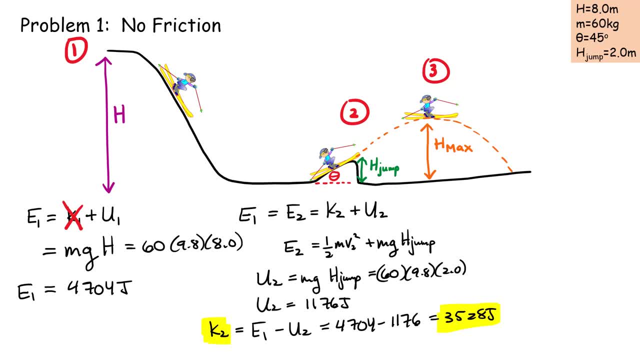 Now, once you know the kinetic energy at any point in the system, you are automatically able to calculate what is the speed, because the kinetic energy at any point in the system is 0.2 mv2.. Okay, The energy at any point in the system is 0.2 mv2 squared. All right, Now let's calculate the kinetic energy. 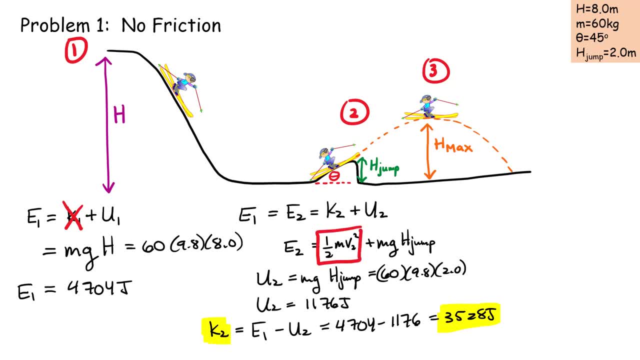 is associated to the speed with this. so all we have now, if you want to find the speed at the top, has to be equal to k2. now I do a little bit of algebra to isolate v2. you bring the two on the other side. divide by the mass and don't. 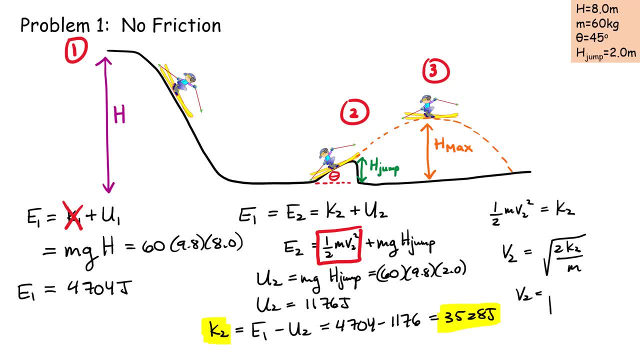 forget to take the square root. now, if you substitute our numbers in here, we get 235, 28 over 60. I put that in the calculator and I get a speed equals to ten point eight of four meters per second. okay, that's how you can find the. 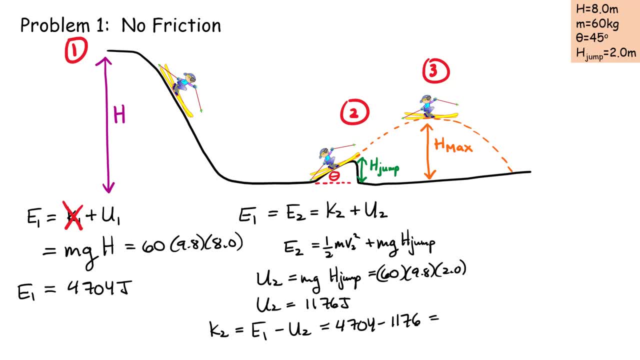 and then minus 1176.. Okay, that gives me a kinetic energy of 3528 joules. Now, once you know the kinetic energy, at any point in the system you are automatically able to calculate what is the speed, because the kinetic energy is associated to the speed. with this, 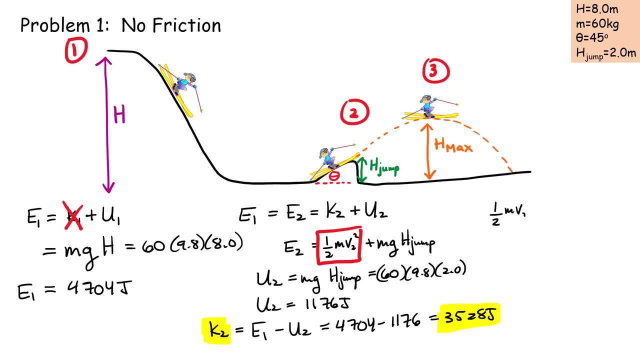 So all we have now is the kinetic energy at the top of this hill. So that gives me a kinetic energy. Now, if you want to find the speed at the top, it has to be equal to k2.. Now do a little bit of. 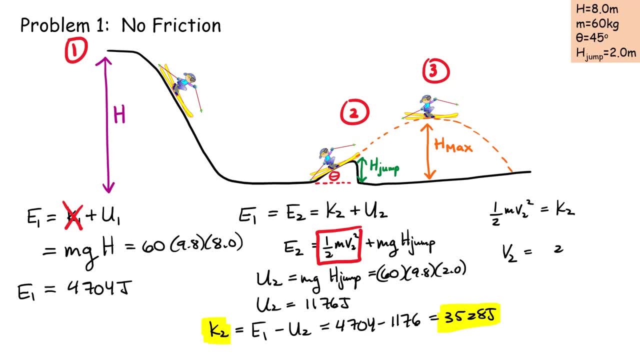 algebra to isolate v2.. You bring the 2 on the other side, divide by the mass and don't forget to take the square root. Now, if you substitute our numbers in here, we get 23528 over 60.. I put. 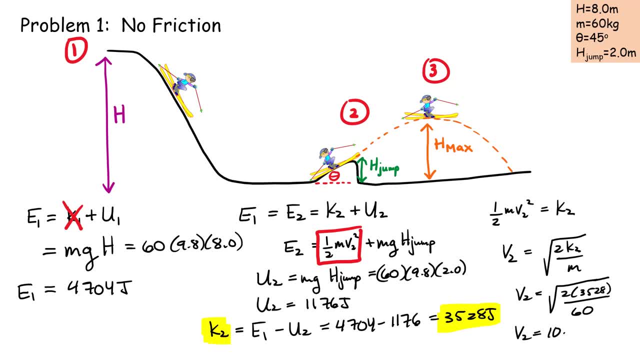 that in the calculator and I get a speed equals to 10.8 of 4.. Okay, that's how you can find the speed here of the skier at the top of the hill, And again, he's launching here at this angle of 45 degrees. Now I just want to highlight a different method. 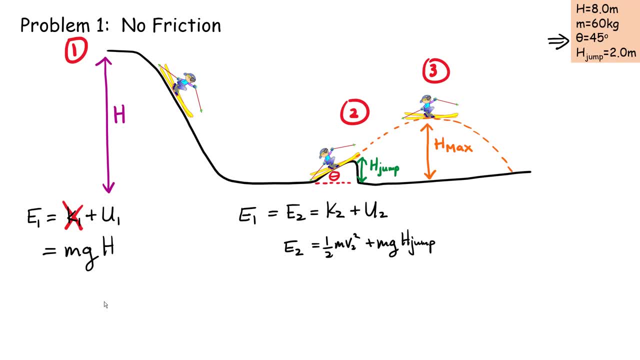 here. What if I didn't substitute in the numbers right away, right? So I have the total energy of the system, which is just simply mgh. right? This here has to be equal to the energy at 0.2 at the. 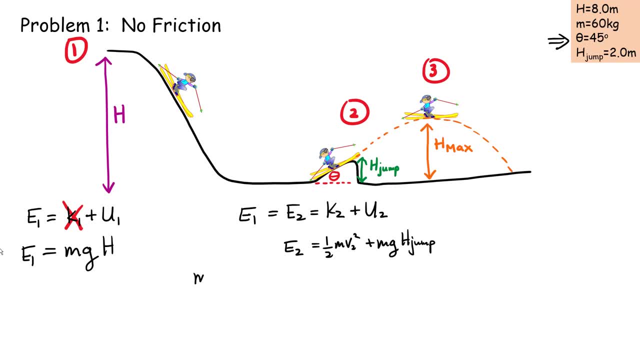 top of the hill. So all you can do now is simply set those equal to k2.. And that's it. So that's equal to each other, right? mgh must be equal to one half mv2 squared plus mgh at the top of the. 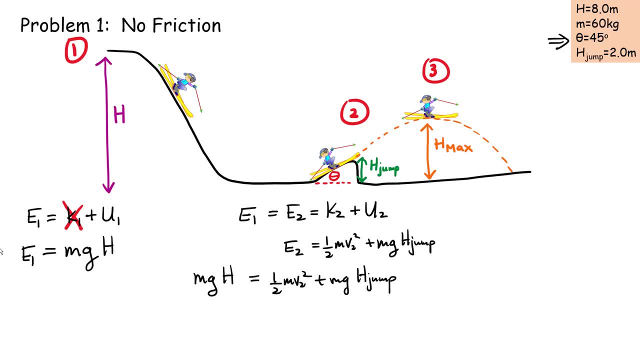 jump Now what you could do now. the only unknown in this equation is actually the speed. So again, if you didn't want to substitute, the other thing you notice is that mass is involved in all the terms, So therefore you can cancel it out. Now. all you have to do is do a little bit of algebra. 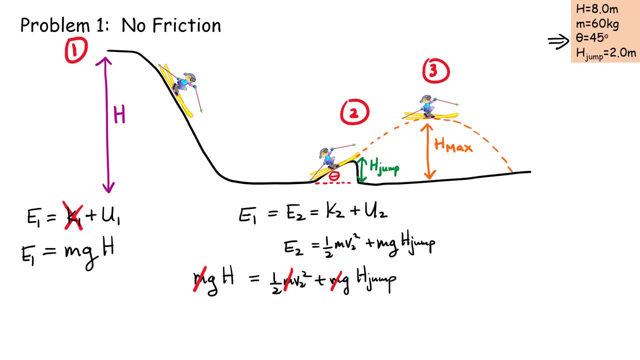 So you bring this gh jump on the other side. I could factor out a, g. it would look like this: right gh minus h jump. What else I can? multiply by two And then, if I take the square root, I'm going to get an expression for v. oops, not v squared, rather v2.. Okay, now you simply go. 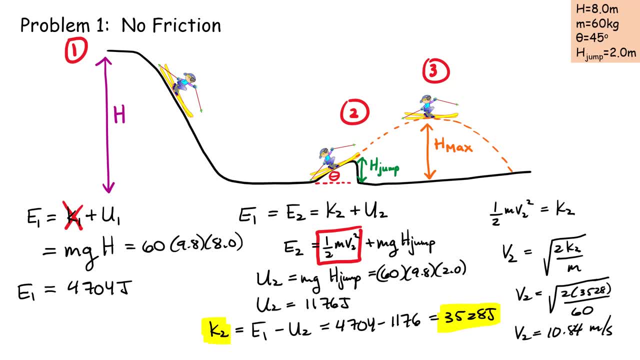 speed here, of the skier at the top of the hill, and again he's launching here at this angle of 45 degrees. now I just want to highlight a different method here. what if I didn't substitute in the numbers, right away? right, so I have the. 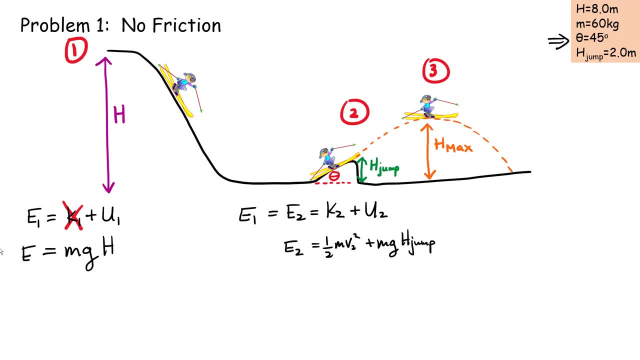 total energy of the system, which is, and just simply, mgh. right, this here has to be equal to the energy at point two, at the top of the hill. so all you can do now is simply set those equal to each other right? mgh must be equal to one half mv2 squared plus mgh. 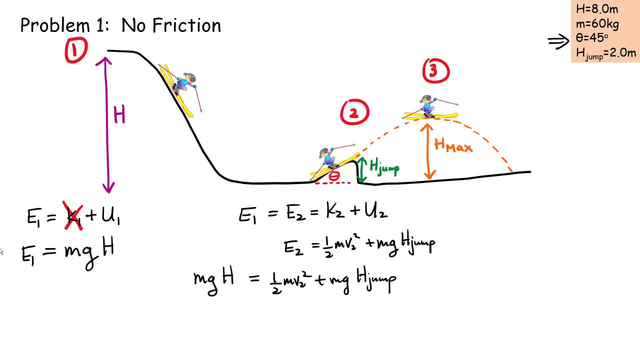 at the top of the jump. now what you could do now. the only unknown in this equation is actually the speed. so again, if you didn't want to substitute, the other thing you notice is that mass is involved in all the terms, so therefore you can cancel it out now. all you have to do is do a little bit of algebra. so 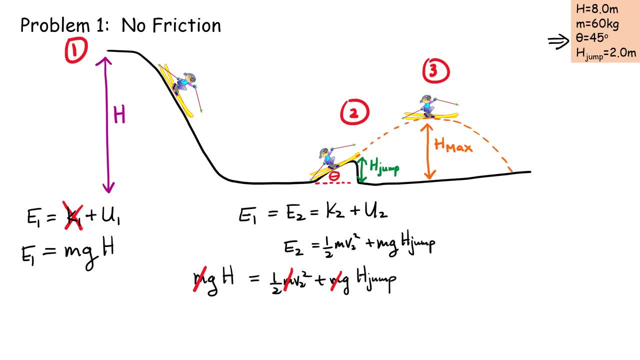 you bring this gh jump on the other side, I could factor out a G. it would look like this: all right, G H minus H jump. what else? I can multiply by two and then, if I take the square root, I'm going to get an expression for V. oops, not V squared, rather V2. 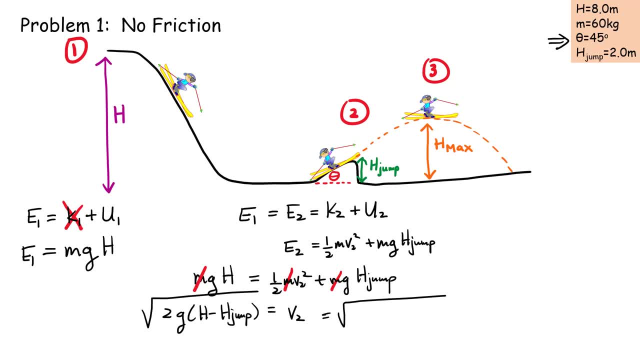 okay, now you simply go through and calculate. you go to nine point eight, and then here you go. eight is the height minus the jump. all right, you put that in your calculator and you're going to get the same answer, okay, of ten point eight, four meters per second. okay, I much prefer this second method. here it takes. 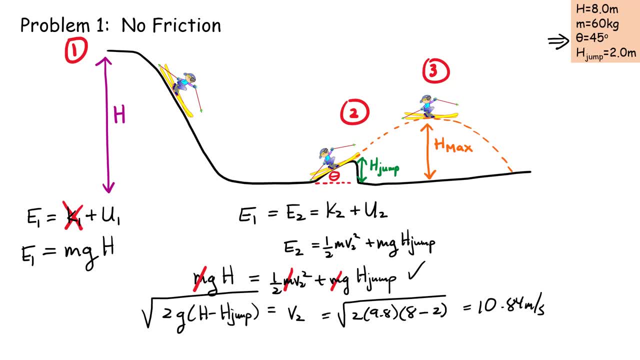 a little bit more algebra, but less likely to make a mistake, I think. all right, so next thing again at the top of this ski jump. here again, I'm assuming a that it's a triangular form, the angle is 45 degrees and that speed we just calculated. is this guy right here? right, it's ten point eight four, but it's. 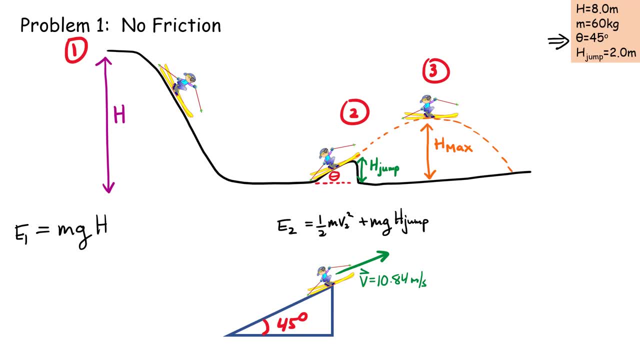 really launching at this angle. so if you form a vector out of that to form a velocity, right, it's not going straight up, it's not going flat, right, you're going off at an angle of 45 degrees. all right, let's now look at the energy at. 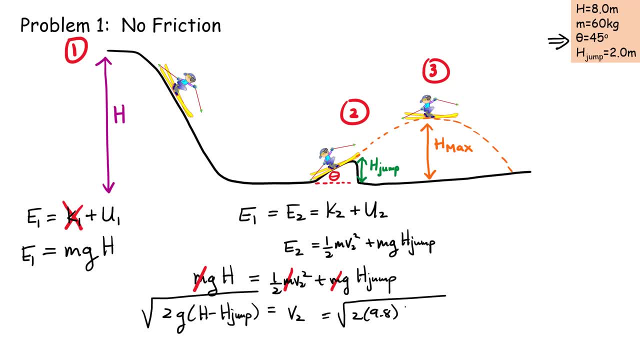 through and calculate, you go to 9.8.. And here you go. eight is the height minus the jump. All right, you put that in your calculator and you're going to get the expression for v, which is the height minus the jump. So you're going to get the expression for v, which is the height minus the. 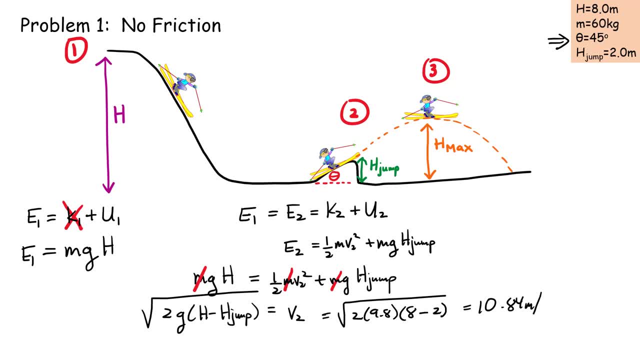 jump. So you're going to get the same answer, okay, of 10.84 meters per second. Okay, I much prefer this second method here. it takes a little bit more algebra but less likely to make a mistake, I think. All right, so next thing again at the top of this ski jump. here again, I'm 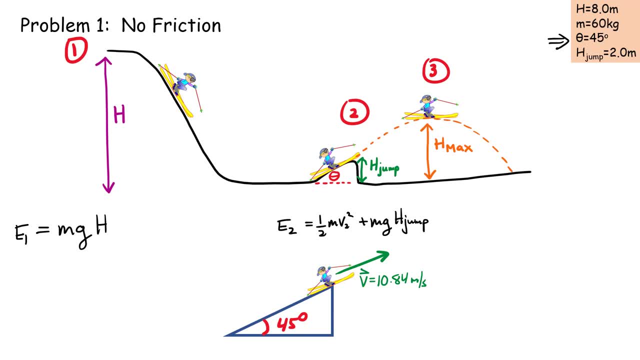 assuming that it's a triangular form. the angle is 45 degrees And that speed we just calculated is this guy right here? right, It's 10.84.. But it's really launching at this angle. So if you form a triangle, you're going to get the same answer. okay, So you're going to get the same. 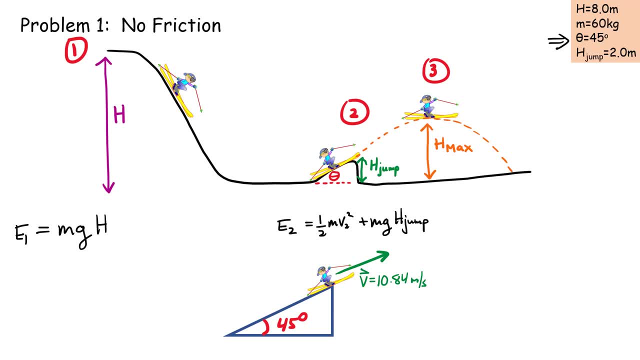 vector out of that to form a velocity, right? It's not going straight up, it's not going flat, right? You're going off at an angle of 45 degrees. All right, let's now look at the energy at the maximum height here. once you launch off this jump, So you write the energy at 0.3.. Again, 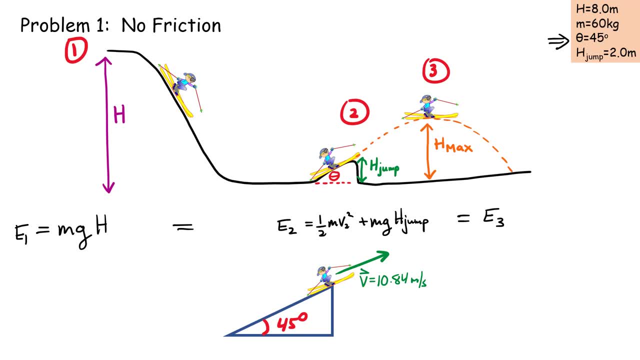 all of these have to be equal because there's no friction anywhere. The energy at the top here. it's still going to have some kinetic energy because I'm still moving right Now. think about what the kinetic energy here is at the top right Now. one thing you know about projectile: 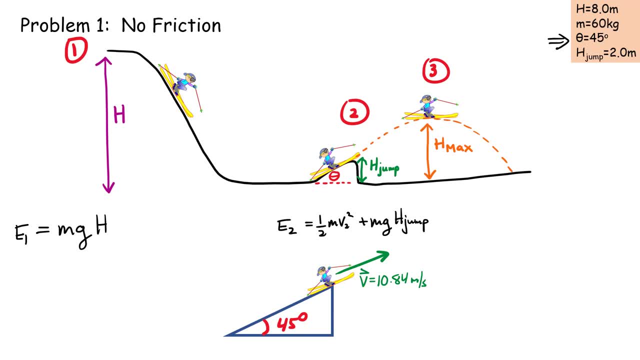 the maximum height here once you launch off this jump. so you write the energy at point three again. all of these have to be equal because there's no friction anywhere. the energy at the top here it's still going to have some kinetic energy because I'm still moving. 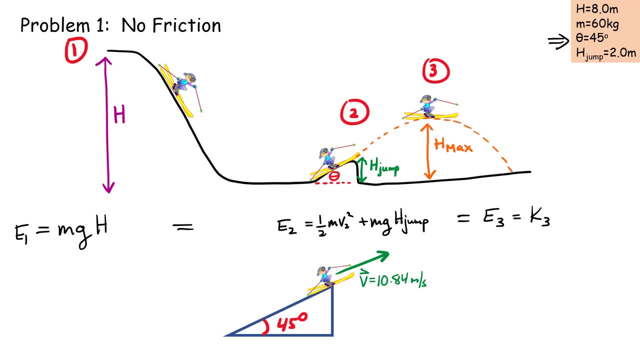 right now. think about what the kinetic energy here is at the top all right now. one thing you know about projectile motion is at the top, all you have is an X component of the velocity, right, you remember V. Y at the top has to be equal to zero, because you kind of you're not moving. 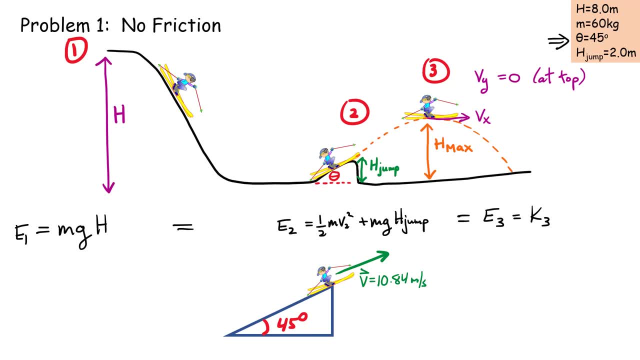 vertically, in a vertical direction, and you're not moving in a vertical direction at the top of that thing, while 30 degrees, all right, all of this is constantly breaking. so if you've한so, it's still coming on from the top. it is not working and you're not raising it. 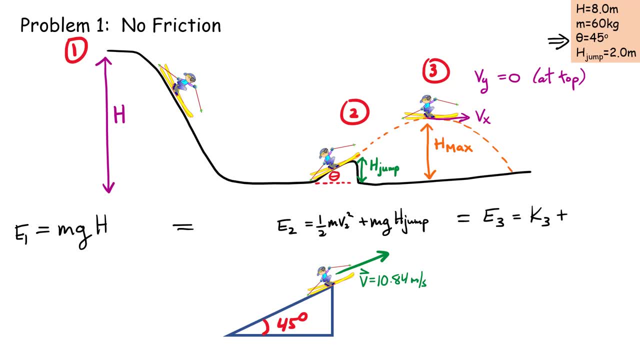 What else? I'm going to be a certain height here above the ground, so I also have some gravitational potential energy, all right. so what do we do? well, we write down our formula for kinetic energy. at the top again, it's VI is zero at the top, but there's still this X component, so I still have some kinetic. 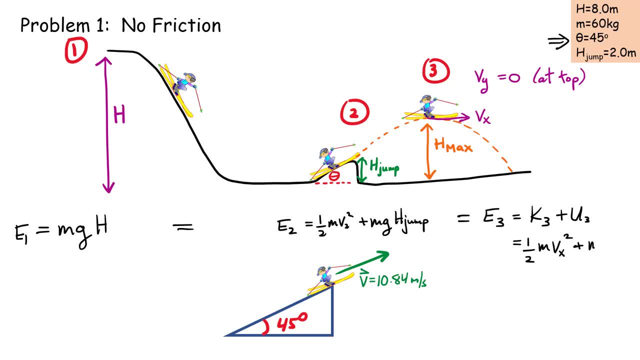 energy at the top plus my gravitational potential energy is MG, and now I'm going to be at this exposio maximum h max, and this is really what i'm trying to solve for that is the total energy at point three. so how do i solve for h max? that was my goal initially for this problem. so do i know the 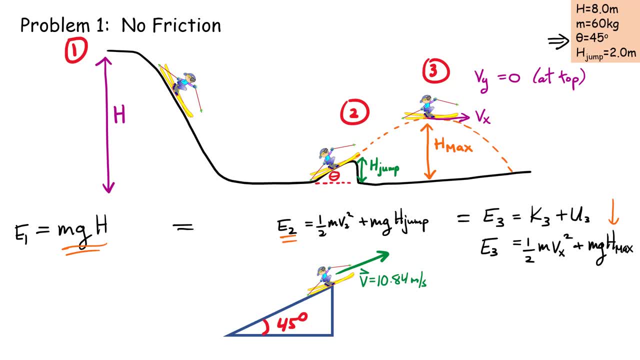 total energy. you bet right, we solved it right here. we solved it over here. we know that value. i need to know what vx is for this problem. how do you solve for vx? so for that you have to go back to 0.2, right? if you have a velocity of 10.84 at an angle of 45 degrees, what you can do is you can. 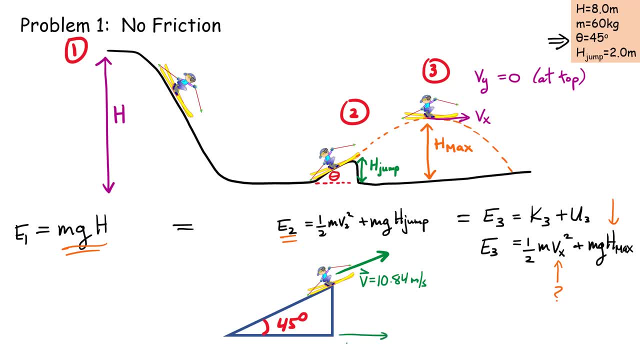 break this down into components. it means it's going to have an x component and it's going to have a y component, right, and that this guy here is the hypotenuse we know is 10.84, so that x component, vx is simply going to be v. multiplied by this is going to be cos of the angle of 45. 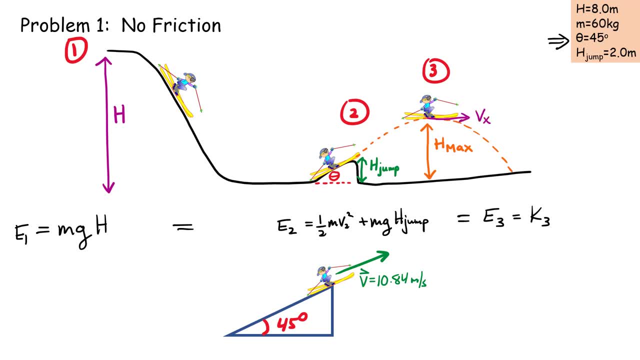 motion is at the top. all you have is an x component of the velocity right. Remember, vy at the top has to be equal to zero because you kind of you're not moving vertically instantaneously at the top of that thing. What else? I'm going to be a certain height here, above. 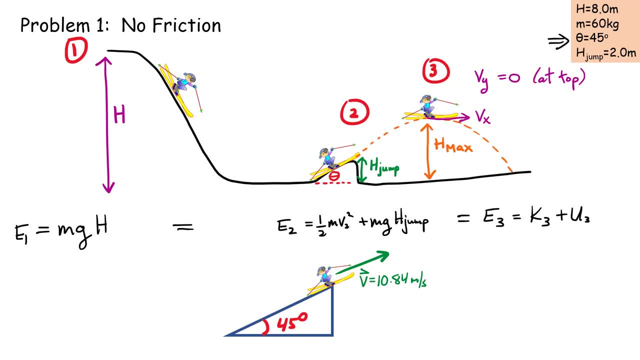 the ground. so I also have some gravitational potential energy. All right, so what do we do? Well, we Write down our formula for kinetic energy at the top. Again, it's vy is zero at the top, but there's still this x component. so I still have some kinetic energy at the top. 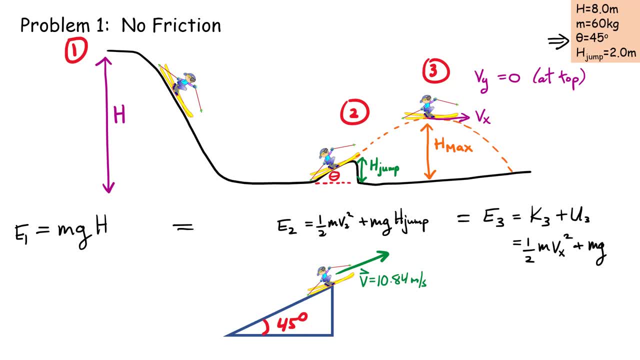 plus my gravitational potential energy is mg, and now I'm going to be at this maximum height, h max, and this is really what I'm trying to solve for. That is the total energy at 0.3.. So how do I solve for h max? That was my goal initially for this. 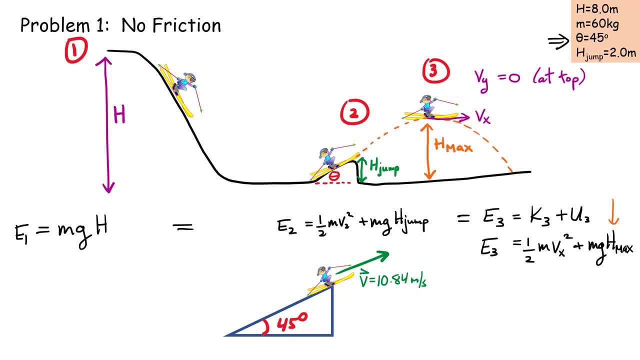 and now I'm going to be at this maximum height, h max, and this is really what I'm trying to solve for. So do I know the total energy? You bet right. We solved it right here. We solved it over here. 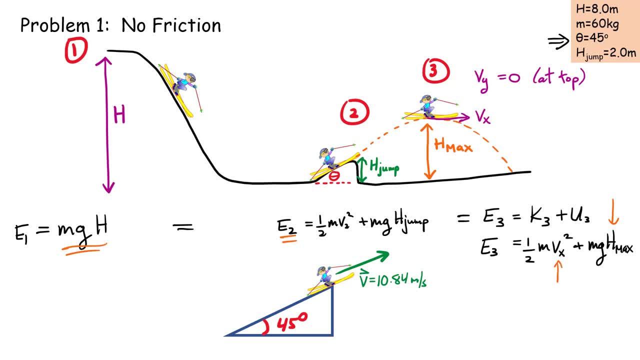 We know that value. I need to know what vx is for this problem. How do you solve for vx? So for that you have to go back to 0.2, right, If you have a velocity of 10.84 at an angle of 45. 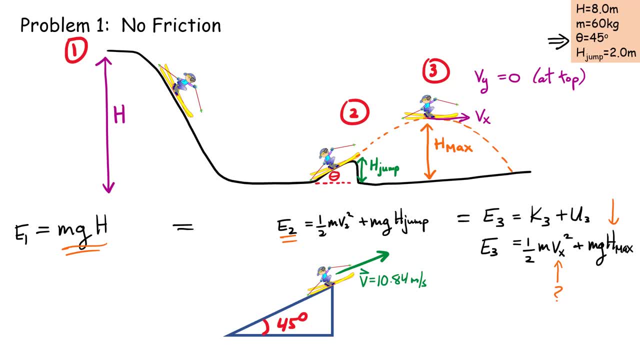 degrees. what you can do is you can break this down into components. It means it's going to have an x component and it's going to have a y component. So what I'm going to do is I'm going to right and that this guy here is the hypotenuse we know is 10.84.. So that x component, vx, is simply: 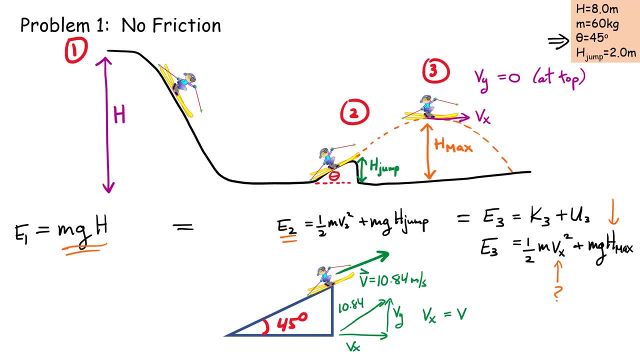 going to be v multiplied by this is going to be cos of the angle of 45 degrees. okay, Now we're going to go ahead and substitute that guy right in here and finish off the math in order to solve for what h max is. So let's go on the next page and continue with this problem. All right now. 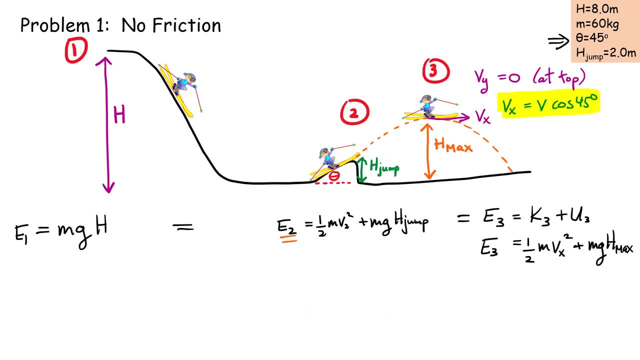 that we know the value of vx. vx doesn't change anywhere in this projectile motion right, It's only the vertical component that changes. What I'm going to do now is I'm going to set well the energy at 0.3, equal to. 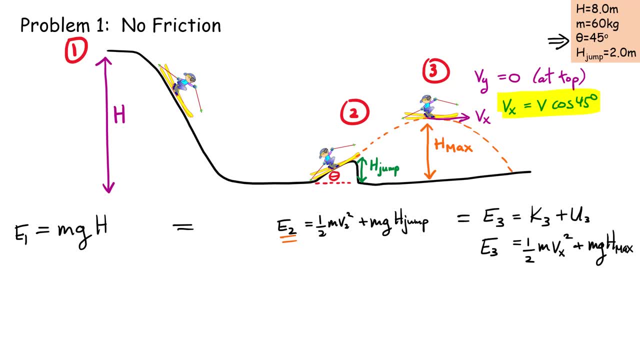 the energy. let me just choose 0.1, since that's kind of the easiest one for me, I think. So we have mgh. the total energy of the system equals to one half m. This is vx squared plus mgh max. 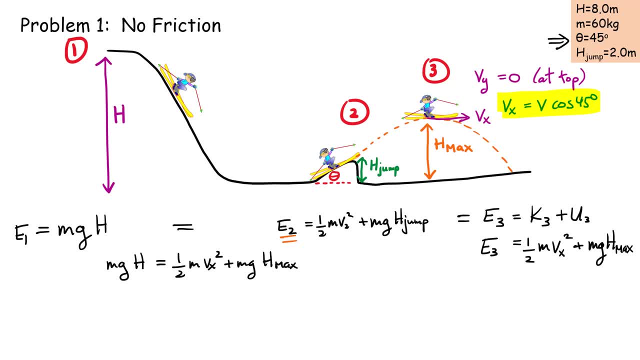 the value that I'm looking for. Again, we have the mass in all the terms. right, Just get rid of it. That simplifies the problem a little bit. Okay, how do I isolate h max here? I can bring this term to the other side, So you have gh. 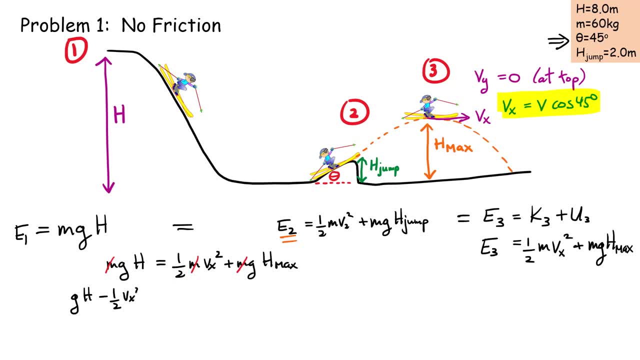 minus one half vx squared equals to gh max. Now, what I'm going to do is divide through by little g, eliminate it from this term, All right. so if you do that, well, you're going to get rid of it here. You're going to get rid of it here, And I have to. 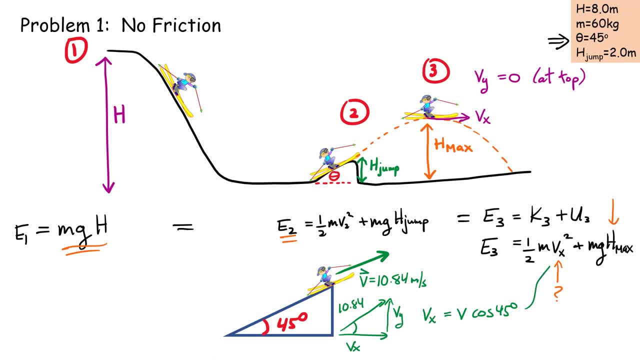 degrees. okay, now we're going to go ahead and substitute that guy right in here and finish off the math in order to solve for what h max is. so let's go on the next page and continue with this problem. all right, now that we know the value of vx, right? vx doesn't change anywhere in this. 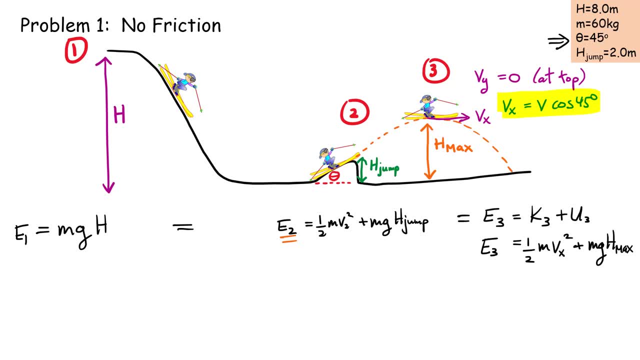 projectile motion. right, it's only the vertical component that changes. what i'm going to do now is i'm going to set, well, the energy at 0.3, equal to the energy. let me just choose 0.1, since that's kind of the easiest one for me, i think. so we have mgh. the total energy of the system equals to one. 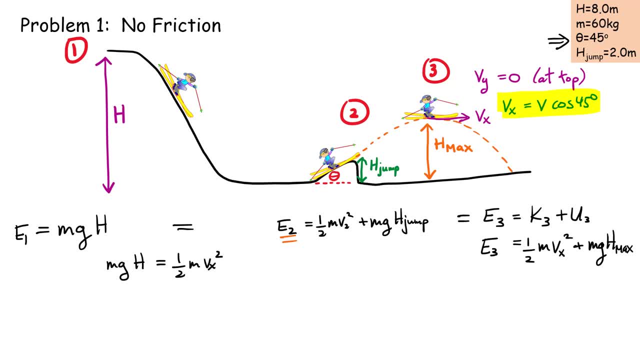 half m. this is vx squared plus mgh max, the value that i'm looking for. again, we have mass in all the terms. right, just get rid of it. that simplifies the problem a little bit. okay, how do i isolate h max here? i can bring this term to the other side, so you have gh minus one half. 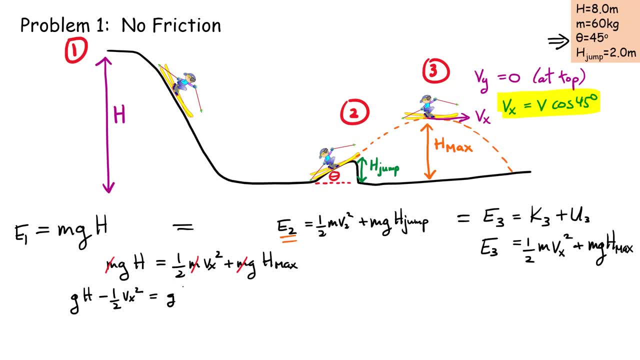 vx squared equals to gh max. now what i'm going to do is divide through by little g. eliminate it from this term, all right. so if you do that, well, you're going to get rid of it here. you're going to get rid of it here and i have to add it to this term divided by little g over here. all right, so we have. 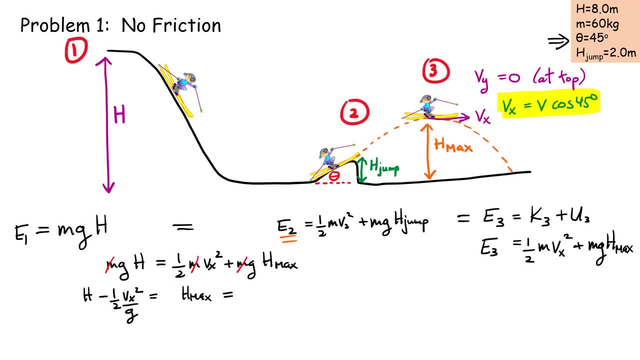 one final expression for h max. all you have to do now is substitute the value. so we have 8.0 for the height, minus one half. now the vx is going to be the value of h max. so we're going to get rid of that. so we're going to have this right. it's v 10.84, cosine of 45 degrees. remember to square that. 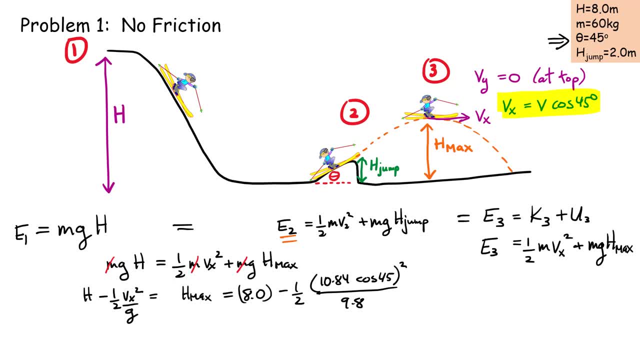 value and divide it by 9.8. okay, so the value of h max that i get for this first problem here is approximately five meters. okay, all right, so that's it for that problem there. pretty straightforward, setting up our equations at the different points and then trying to get to an expression for h max. 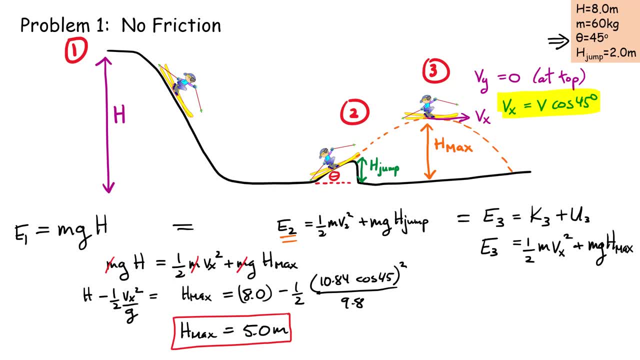 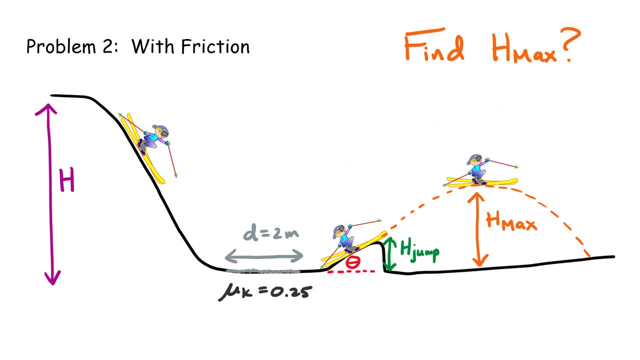 max. let's see how the problem changes now if i introduce friction in this middle section. all right, here's problem two. now what we're gonna do is we're gonna add a little bit of friction over here, just in this flat section- um kind of a rough patch in the snow. here i'm going to give 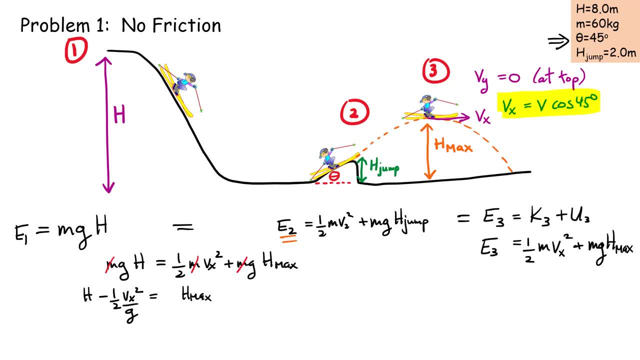 add it to this term divided by little g over here. All right, so we have one final expression for h max. All you have to do now is substitute the value, So we have 8.0 for the height minus one half. Now the vx is going to be this right: It's v 10.84, cosine of 45 degrees. 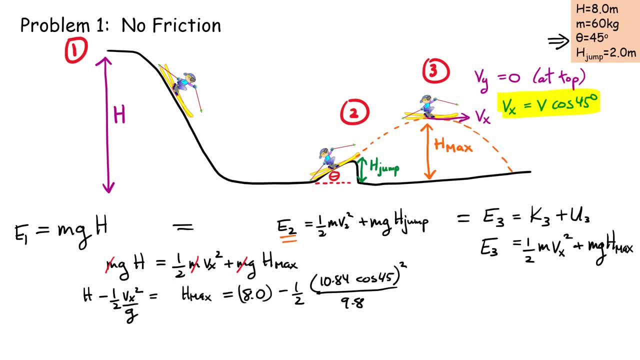 Remember to square that value and divide it by 9.8.. Okay, so the value of h max that I get for this first problem here is approximately five meters. Okay, All right, so that's it for that problem there. Pretty straightforward setting up our equations at the different points. 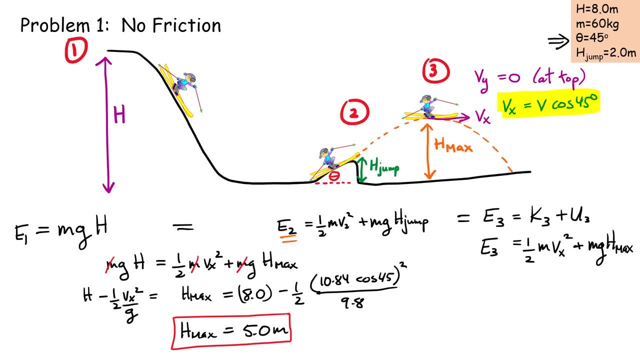 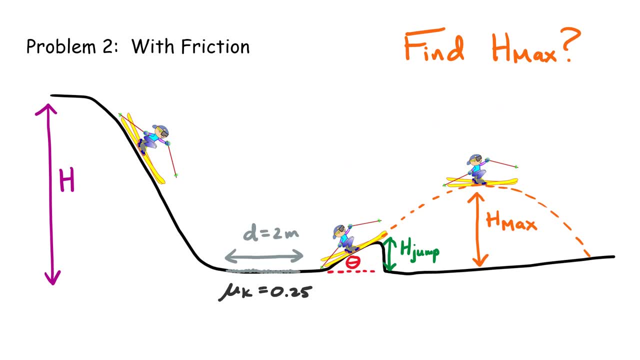 and then trying to get to an expression for h max. Let's see how the problem changes now. if I introduce friction in this middle section, All right, here's problem two. now, What we're going to do is we're going to add a little bit of friction over here, just in this flat section. 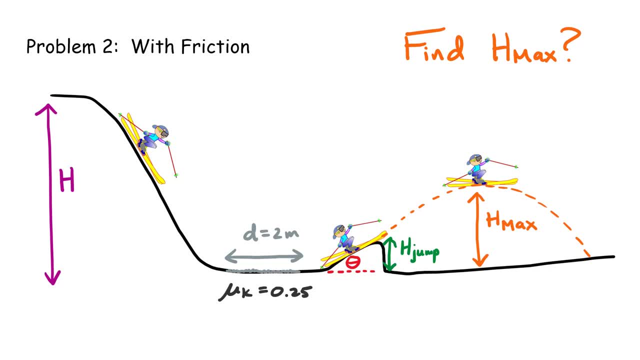 kind of a rough patch in the snow. here I'm going to give you the coefficient of kinetic friction here between the skis and the snow and this distance here that is going to slide over this friction patch. Again, my goal is to calculate. 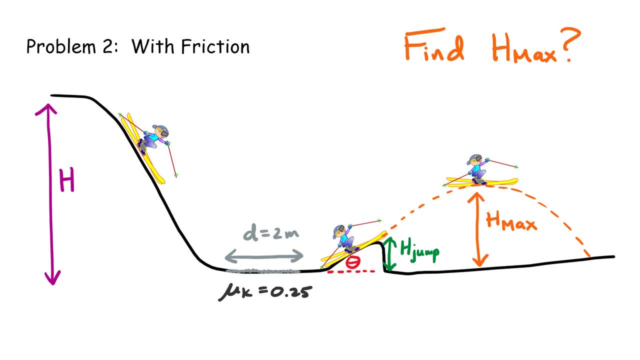 what is this maximum height? and we're going to use the concept of energy. But let's first look at what's going on. when he's in this middle section here, All right, if you look at kind of the skier when he's sliding across, well, what forces do we have? Well, we have the weight acting down right. 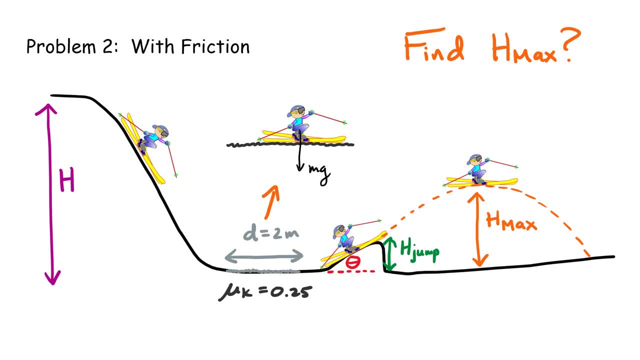 mg. There's the snow pushing up on him. so there's this kind of normal force here. n And now, since there is kinetic friction here, what we have to do is we have to add this force right here. This is going to be a friction force of kinetic friction. It opposes the motion right. Keep in. 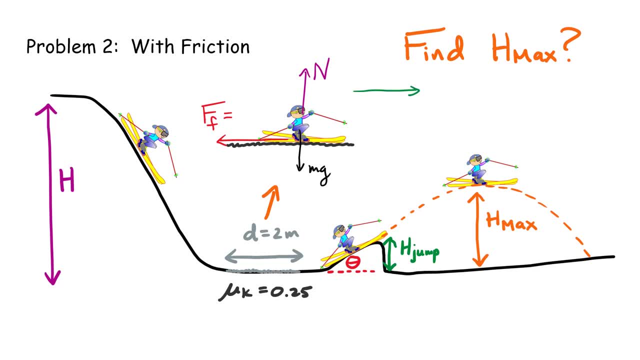 mind. he is moving, He's moving in this direction. He's moving a distance d right. That is going to be his displacement. Displacement delta x. it's just going to call it d, but it's actually. it's a vector that is going to the right, The force of friction. if you remember from your class, 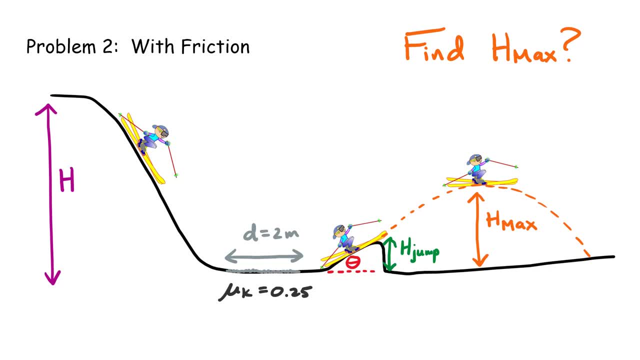 you the coefficient of kinetic friction here between the skis and the snow and this distance here that is going to slide over this friction patch again, my goal is to calculate what is this maximum height? um, and we're going to use the concept of energy, but let's first look at what's. 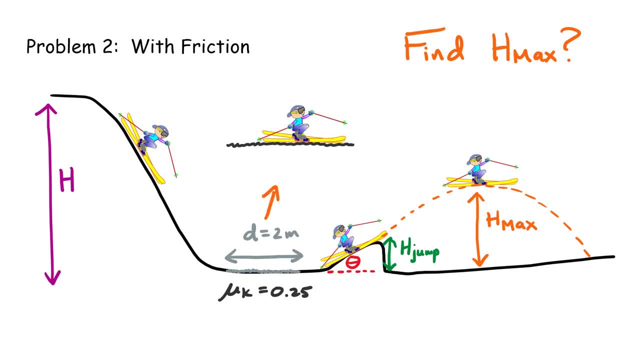 going on when he's in this middle section, here, right, if you look at kind of the skier, when he's sliding across. well, what forces do we have? well, we have the weight acting down right, mg, what else? there's the snow pushing up on him. so there's this kind of normal force here, n and now since 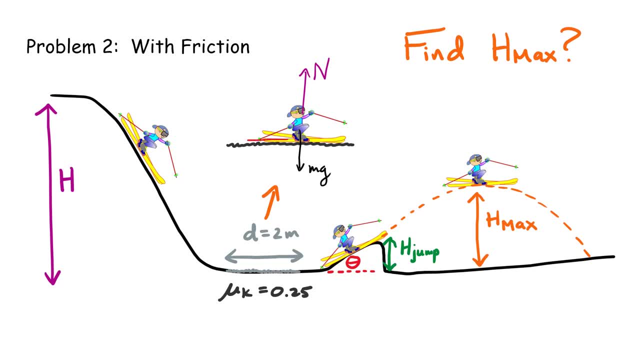 there is kinetic friction here. what we have to do is we have to add this force right here, here. this is going to be a friction force of kinetic friction. it opposes the motion. right, keep in mind, he is moving. he's moving in this direction. he's moving a distance d right that. 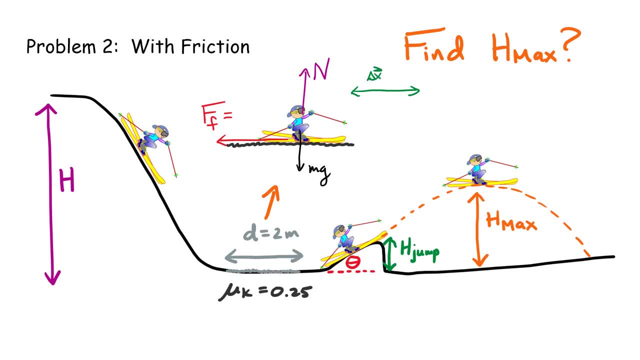 is going to be his displacement. displacement delta x. it's just going to call it d, but it's actually a vector that is going to the right. the force of friction: if you remember from your class, you can write that as a coefficient of kinetic friction multiplied by the normal. 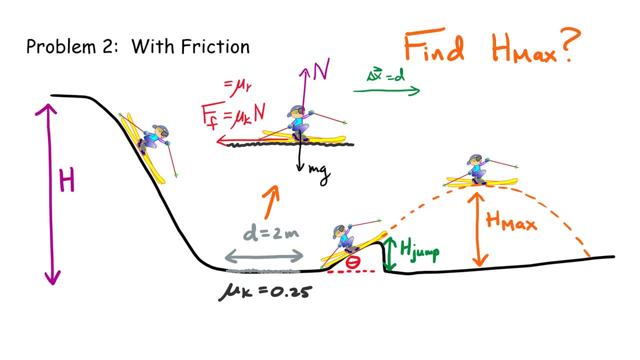 force, and in this case the normal force is simply equal to the weight these forces here balance out when he's on a flat section. so you know this force here of kinetic friction, so we can now calculate how much energy is being lost as he goes over this rough patch. 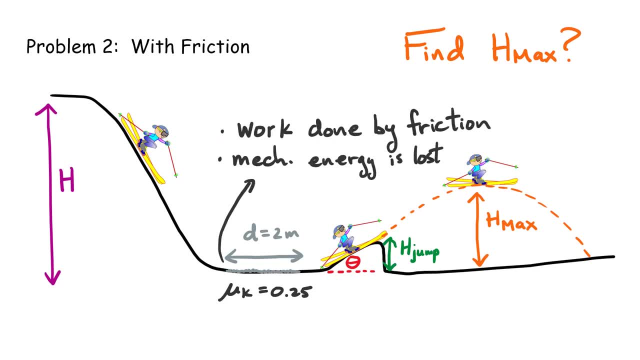 right, because, guess what? there is going to be work done by this friction force, and whenever there's work done by the force of friction, that means that some of the mechanical energy is going to be dissipated as heat. it's going to be mechanical energy that's lost, okay. so how do we account for this? so, basically, 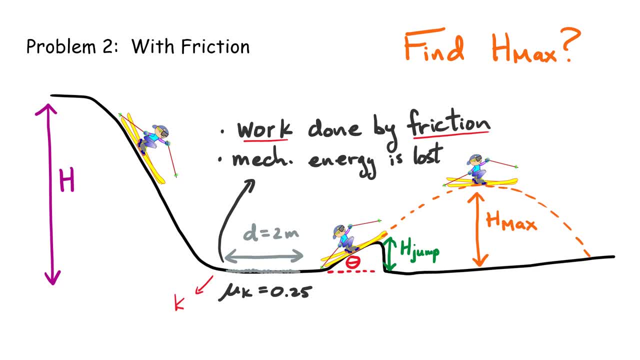 if you calculate how much kinetic energy there is here at the beginning, right? if you call that, say, k beginning versus k end, these guys can't be the same, right? these values can't be the same because i've lost some energy due to friction. so let's go ahead and set up the equation. 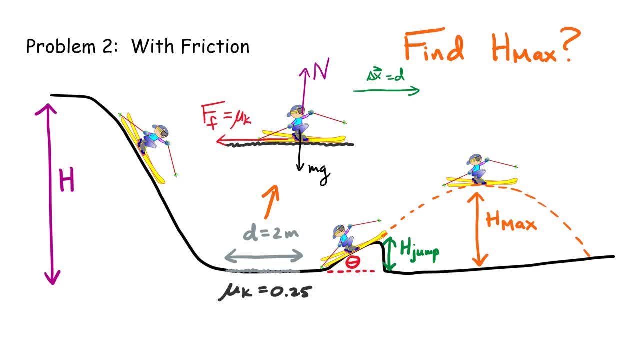 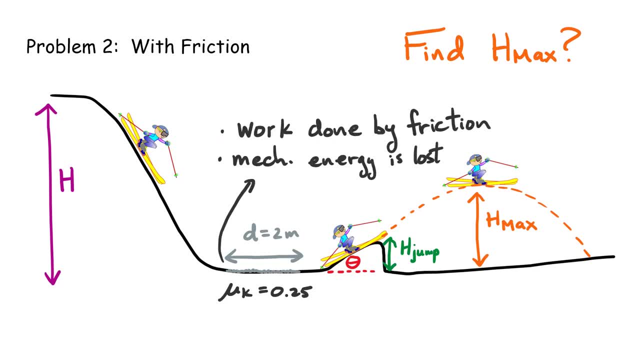 So we can now calculate how much energy is being lost as he's sliding across. So we can now calculate how what There is going to be work done by this friction force. And whenever there's work done by the force of friction, that means that some of the mechanical energy is going to be dissipated. 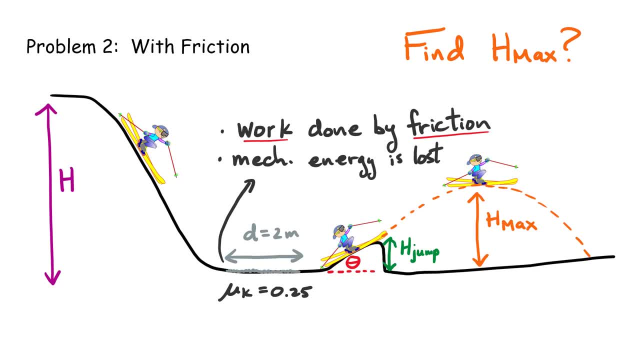 as heat. It's going to be mechanical energy that's lost, Okay, so how do we account for this? So, basically, if you calculate how much kinetic energy there is here at the beginning, right, if you call that, say, K beginning versus K end, these guys can't be the same, right, These values? 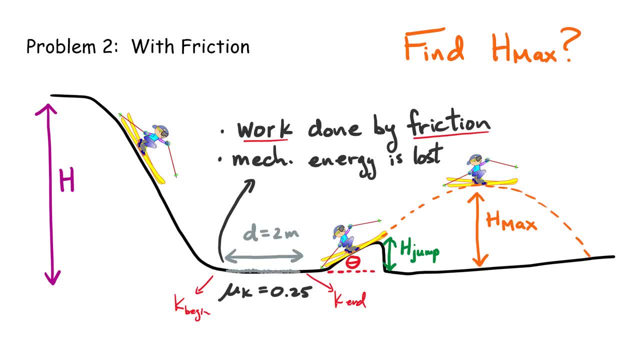 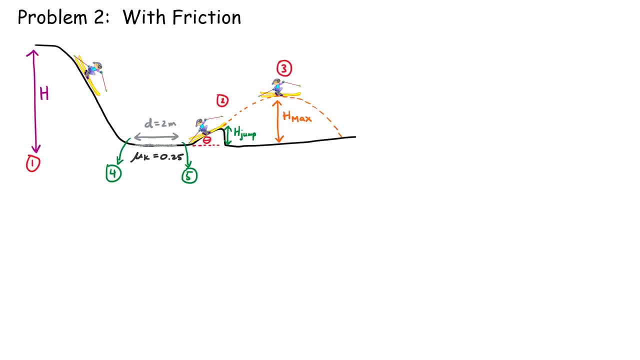 can't be the same, because I've lost some energy due to friction. So let's go ahead and set up the equations now and redo this problem with friction. All right, so to solve this problem, we're going to define the points just like we did before. We have points one, two and three, So one. 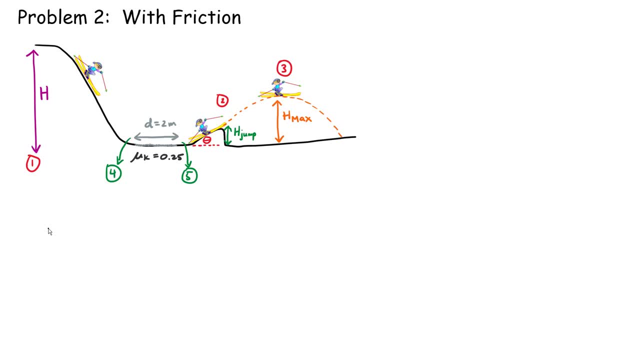 was at the top of the hill, two top of the jump and three at the top of at the maximum height. I've added two points here just to illustrate how we're going to set up the equations. Point four is right before I hit the rough patch. Point five is right after I hit the 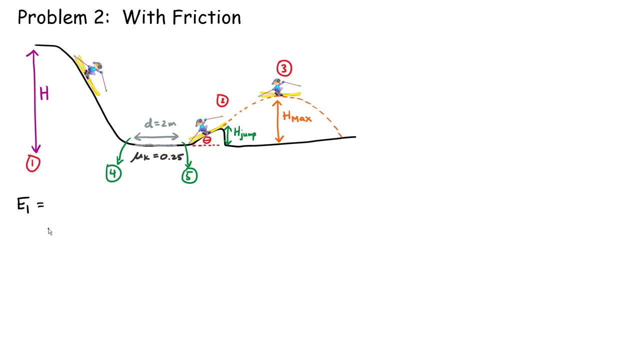 rough patch. So the energy at point one- you would simply write it as the kinetic energy at point one plus the gravitational potential energy at point one, And this guy is zero again, because I'm starting very, very slowly or starting at rest. So that means that this guy is simply MGH. 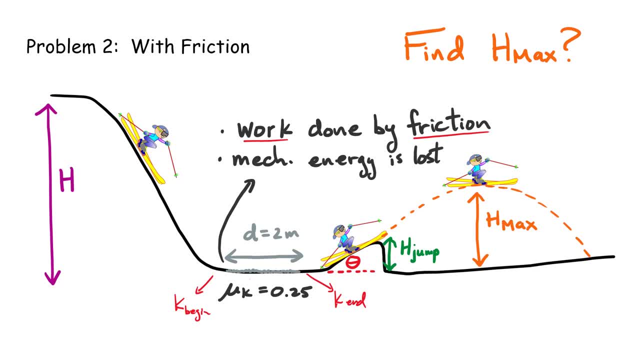 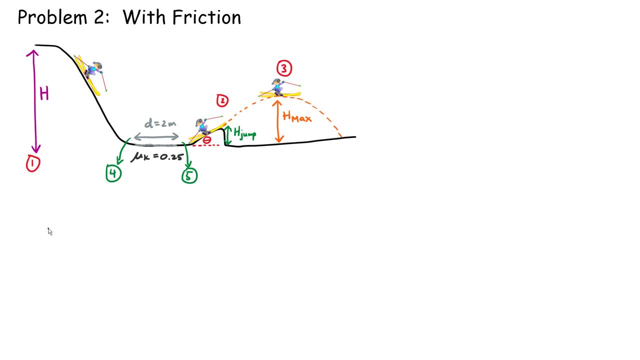 now and redo this problem with friction. all right, so to solve this problem, we're going to define the points just like we did before. uh, we have points one, two and three. so one was at the top of the hill, two top of the jump and three at the top of at the maximum height. i've added two points here. 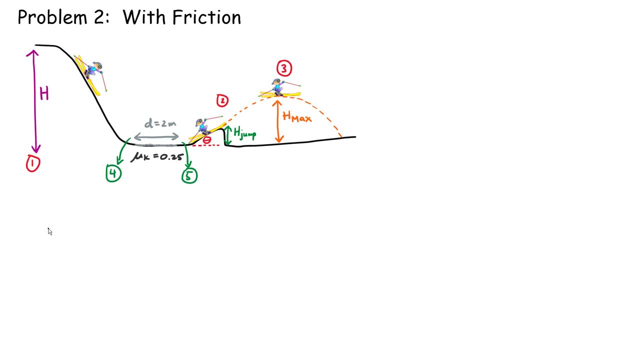 just to illustrate how we're going to set up the equations: 0.4 is right before i hit the rough patch. 0.5 is right after i hit the right, the rough patch. so the energy of 0.1, you'd simply write it as the. 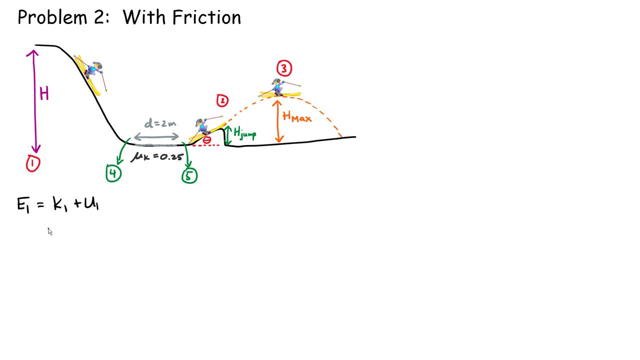 the kinetic energy at 0.1 plus the gravitational potential energy at 0.1. And this guy is zero again, because I'm starting very, very slowly or starting at rest. So that means that this guy is simply MGH- the height of the hill, just like we did before. we calculated that value. We know what? 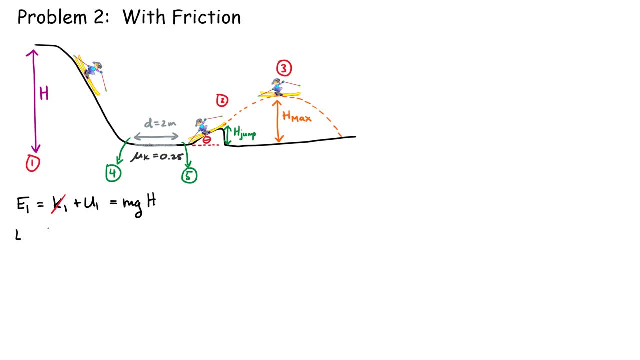 that is Now the energy at 0.4,. let me go ahead and write that guy. So again, it's going to be the kinetic energy at 0.4 plus the gravitational energy at 0.4.. Okay, Now there is another. 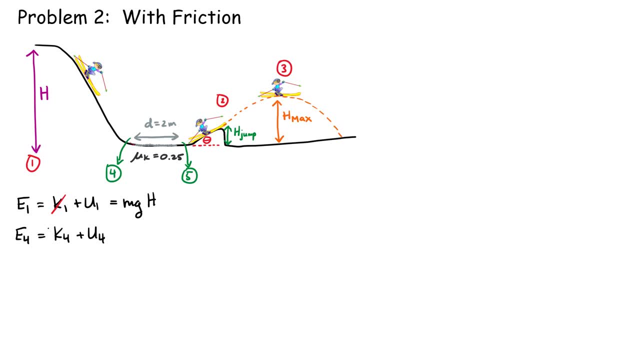 simplification, that happens at 0.4, because, since I'm on the flat surface over here, there is no gravitational potential energy. So guess what? That means that over here, all I have is kinetic energy. I haven't lost any energy yet. right, I'm converting all of this gravitational potential. 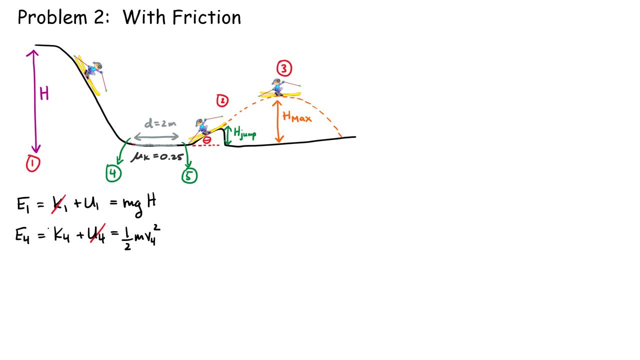 energy into kinetic energy. Well, guess what I can find, how fast I can convert all of this gravitational potential energy into kinetic energy. I'm moving over here at 0.4.. That would be very straightforward: I simply equal the energy at. 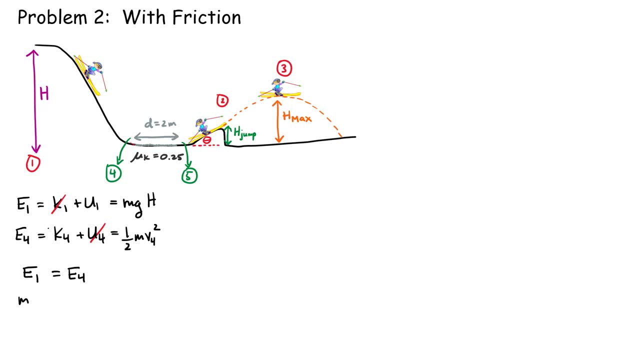 0.1 to the energy at 0.4.. I haven't lost anything. So you get MGH equals to one half MV4 squared Again. the masses cancel out. That's kind of helpful, And at the end you get an expression. 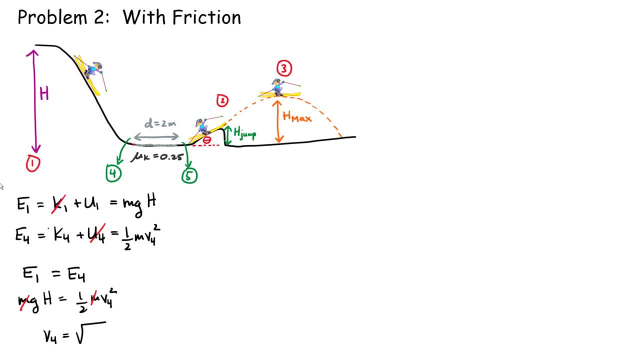 for V4, which is simply the root of two times little g times the height- Okay, I can find how fast I'm moving right here. So two, 9.8, and the height was eight meters, same as before. Put that in the calculator and, lo and behold, we get 12.52 meters per second. All right, So that's. 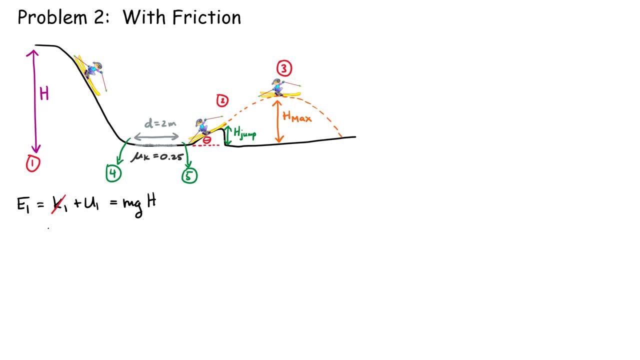 the height of the hill, just like we did before. we calculated that value. We know what that is Now. the energy at point four. let me go ahead and write that guy. So again, it's going to be the kinetic energy at point four plus the gravitational energy at point. 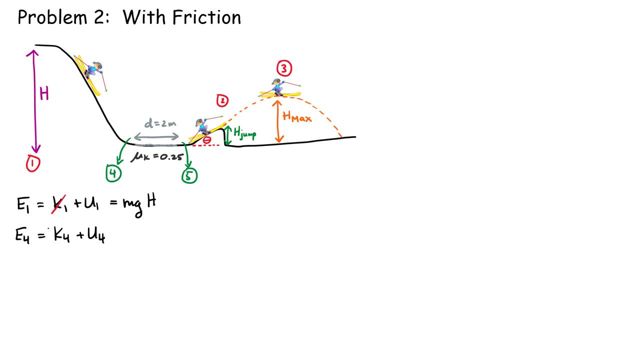 four. Okay, Now there is another simplification. that happens at point four, because since I'm on the flat surface over here there is no gravitational potential energy. So guess what? That means that over here all I have is kinetic energy. I haven't lost any energy yet, right? 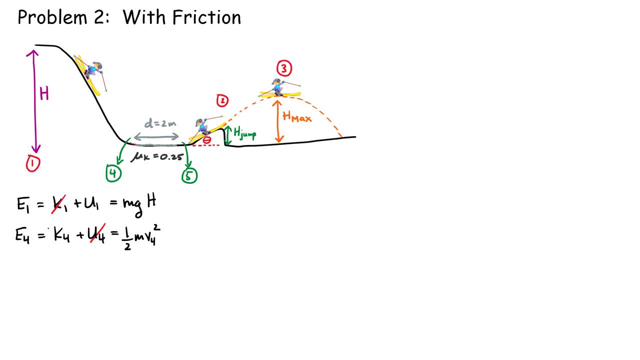 I'm converting all of this gravitational potential energy into kinetic energy. Well, guess what? I can find how fast I'm moving over here at point four. That would be very straightforward. I simply equal the energy at point one to the energy at point four. I haven't. 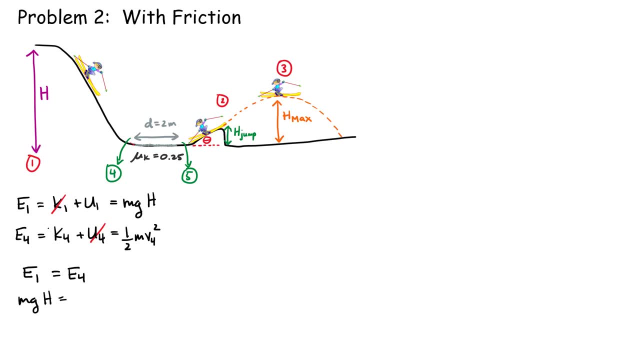 lost anything. So you get MGH equals to one half MV4 squared Again. the masses cancel out That's helpful And at the end you get an expression for V4, which is simply the root of two times little g times the height. Okay, I can find how fast I'm. 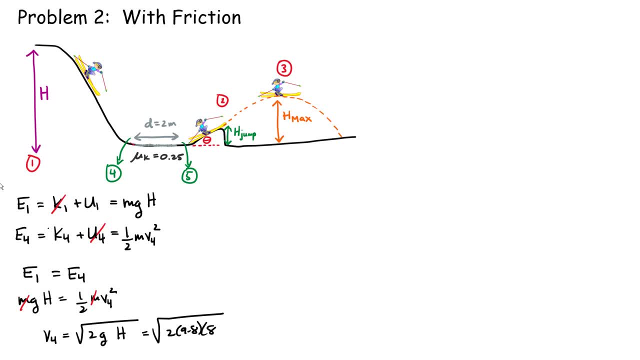 moving right here. So two, 9.8, and the height was eight meters, same as before. Put that in the calculator and, lo and behold, we get 12.52 meters per second. All right, So that's how fast. 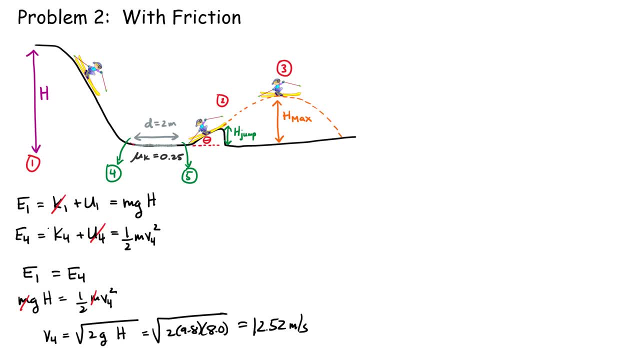 I'm moving before I hit the rough patch. Okay, Now how do we deal with losing speed over here, through the rough patch, using energy? Now you can't write this statement. Let's make sure we understand here that the total mechanical energy at four, you wouldn't be able to write this. 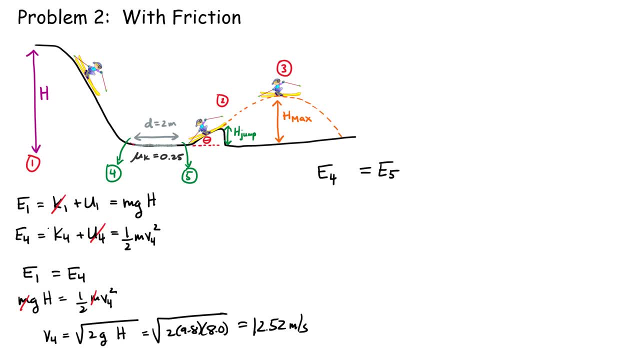 statement right here. right, Because if you did that, you would actually end up having the same speed. right, Because there is no gravitational potential energy at point four. There is none at point five. So we really can't do this right. Mechanical energy is not going to be conserved. 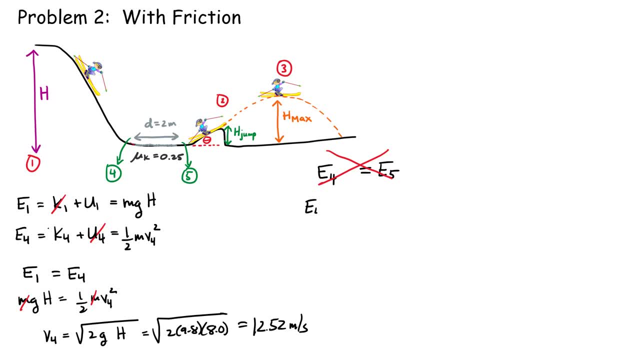 here. So what we have to do is: you have to do that. You have to have a mechanical energy at point four to do something like this. the energy at point four is actually going to be bigger than the energy at point five. okay, what we have to do now is: you have 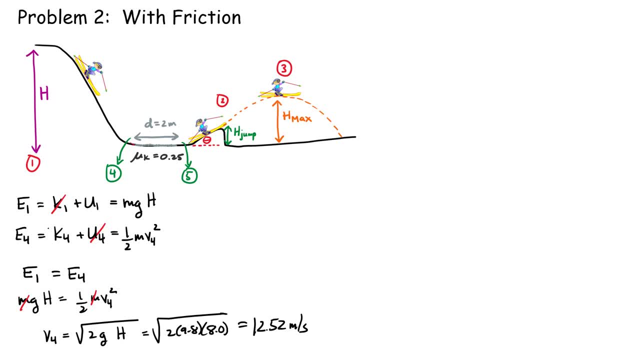 how fast I'm moving before I hit the rough patch. Okay, Now how do we deal with losing speed over here through the rough patch, using energy? Now you can't write this statement. Let's make sure understand here that the total 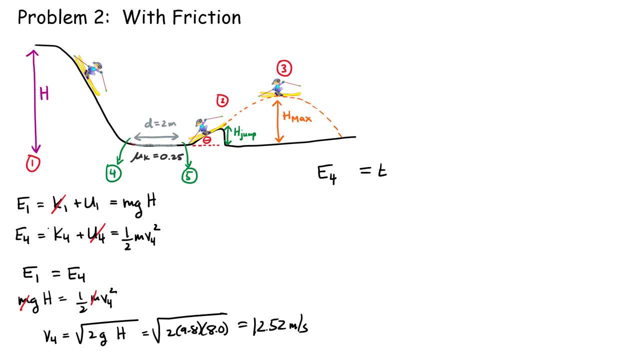 mechanical energy at four, you wouldn't be able to write this statement right here. right, Because if you did that, you would actually end up having the same speed. right, Because there is no gravitational potential energy at 0.4.. There is none at 0.5.. So we really can't do this right. 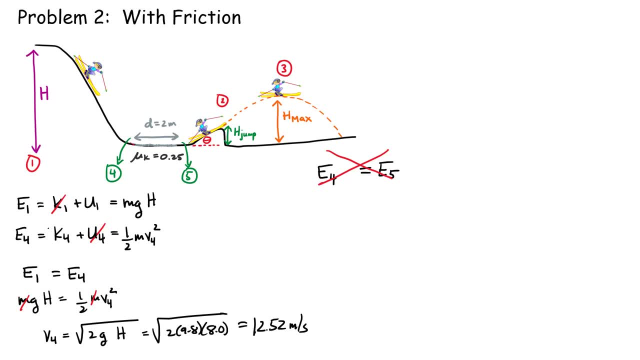 Energy is mechanical. energy is not going to be conserved here, So what we have to do is you have to do something like this: The energy at 0.4 is actually going to be bigger than the energy at 0.5.. Okay, What we have to do now is you have to add the work done by any non-conservative force. 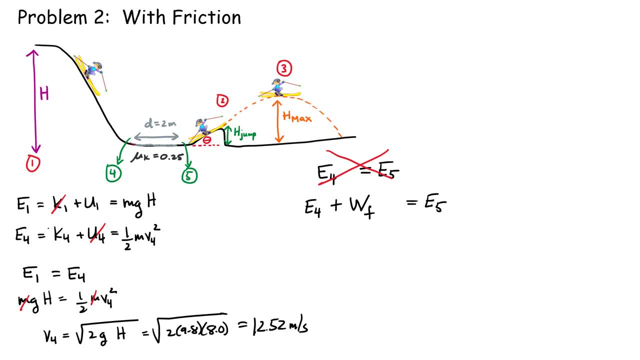 So in this case, a non-conservative force is the work done by friction. So remember our free body diagram. here we had all our forces labeled on it, And if I wanted to calculate how much work is done by this friction force, again, you simply apply a formula: It's the force multiplied by the. 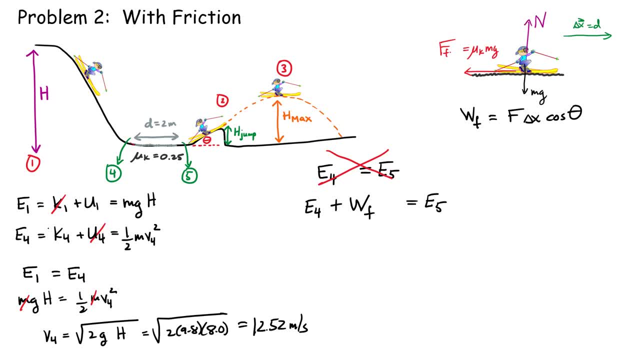 displacement multiplied by cos of the angle, And then you multiply that by the force multiplied by the force multiplied by the displacement multiplied by cos of the angle, And then you multiply that by the force multiplied by the angle between the force and the displacement. In. 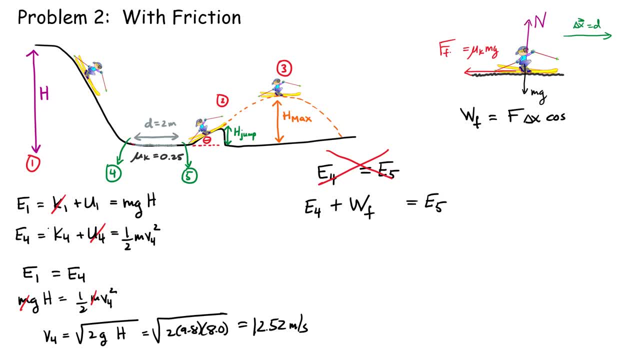 this case the angle is going to be 180 degrees right, Because the force is acting to the left and my displacement vector is to the right and cos of 180 is minus one. So this guy here is simply minus the magnitude of the force of friction multiplied by the magnitude of the displacement which, in 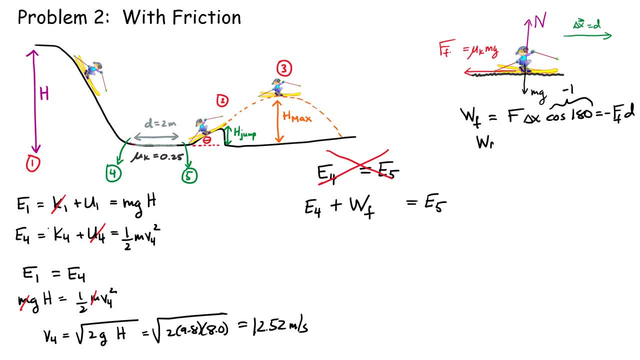 this case is just D. All right, So you can get a number for this right: The work done by force of friction minus mu KMG multiplied by D. All right, You put the numbers in the calculator. you get minus 0.25.. That was the coefficient of friction. The mass was 60. This was 9.8.. And my displacement? 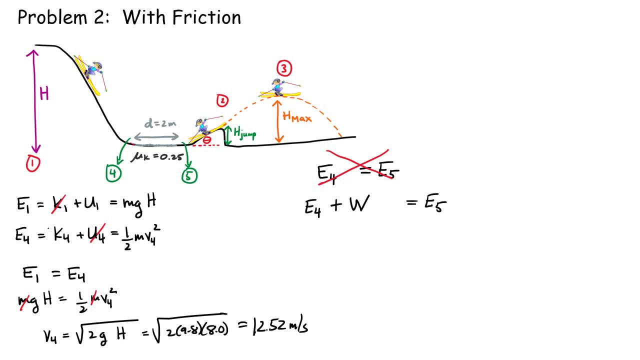 to add the work done by any non conservative force. so in this case, a non conservative force is the work done by friction. so remember our free body diagram. here we had all our forces labeled on it, and if I wanted to calculate how much work is done by this friction force, again, you simply apply a. 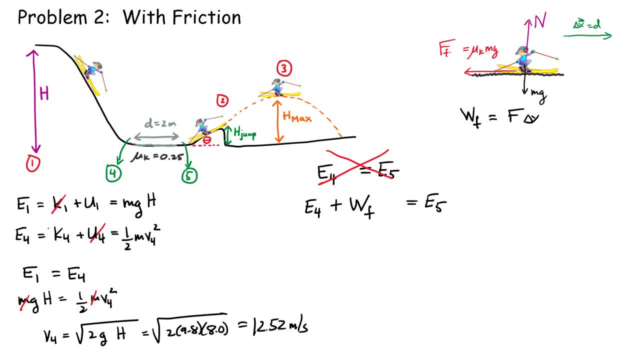 formula. it's the force multiplied by the displacement, multiplied by cos of the angle between the force and the displacement. in this case, the angle is going to be a hundred and eighty degrees. all right, because the force is acting to the left and my displacement vector is to the right and cos of 180 is minus one. 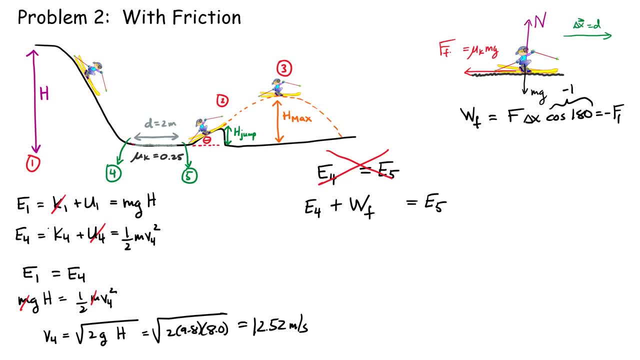 so this guy here is simply minus the magnitude of the force of friction multiplied by the magnitude of the displacement, which in this case is just the force acting to the left, and my displacement vector acting to the right is d all right, so you can get a number for this right. the work done by force of 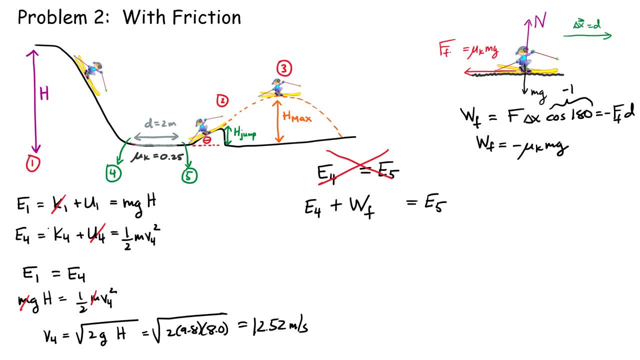 friction minus mu K mg multiplied by D. all right, you put the numbers in the calculator. you get minus 0.25. that was the coefficient of friction. the mass was 60, this was 9.8 and my displacement is 2 and my work done by the force of. 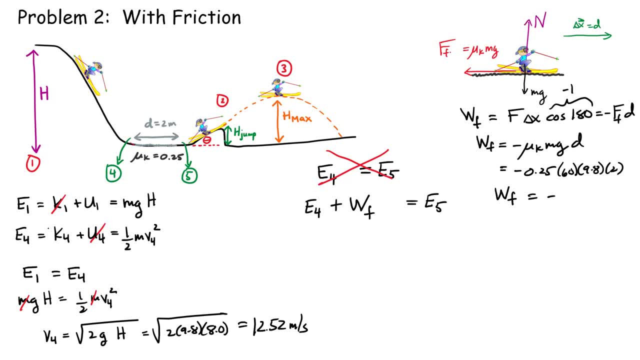 friction. for this case, again, I get a negative value minus 294 joules. so that means we took 294 joules of mechanical energy out of the system. so how much energy then do I have left here at 0.5? well, again we started with what. 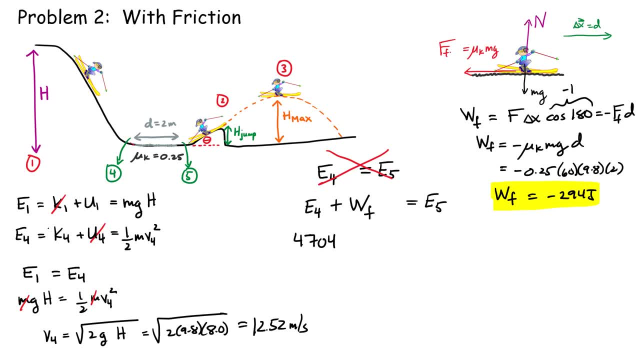 was the number, we had 4704, and now, if I put the work done by friction, 294, this is my energy at point five. the energy at point five is the kinetic energy at point 0.5 plus the gravitational potential energy at 0.5, but since we're on the flat surface, it's simply. 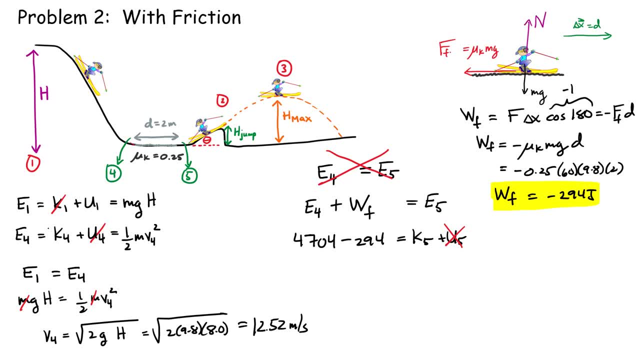 the kinetic energy at 0.5, which gives me a value of 4410 joules. that's the kinetic energy over here at 0.5. well, let me just kind of get rid of the unit here. um, just call that k5. well, let's put it. 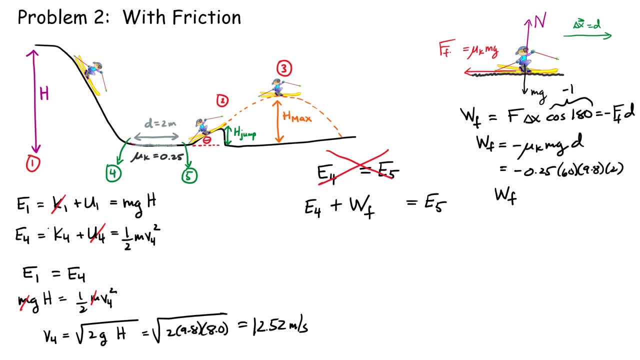 is two And my work done by the force of friction. for this case again, I get a negative value minus 294 joules. So that means we took 294 joules of mechanical energy out of the system. So how much energy then do I have left here at 0.5? Well, 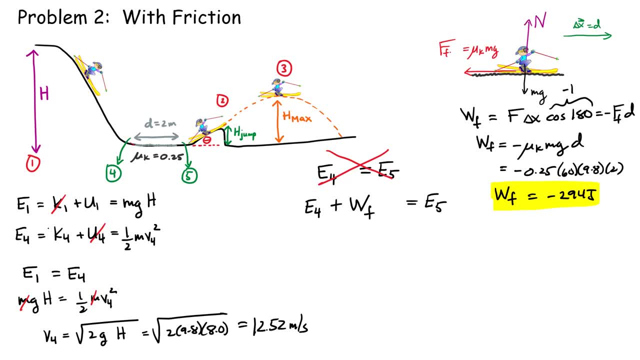 again. we started with what was the number. We had 4,704.. And now, if I put the work done by friction, 294, this is my energy at 0.5.. The energy at 0.5 is the kinetic energy at 0.5 plus. the gravitational potential energy at 0.5.. But since we're on the flat surface, you get 10.3 Joules. You can get a negative value of the force of friction. We're taking the large energy here And now. I'm taking the small energy and I'm taking the small energy, I'm taking the large energy. 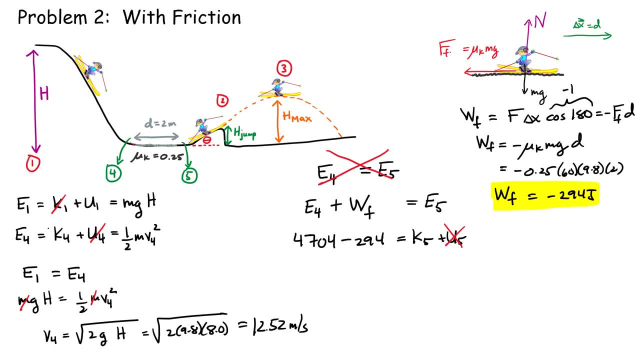 and I'm taking the small energy, I'm taking the medium, I'm taking the small energy And I'm taking the large energy And I'm taking the medium And I'm taking the medium. But again, you can do the, since we're on the flat surface. it's simply the kinetic energy at 0.5, which gives me a value of 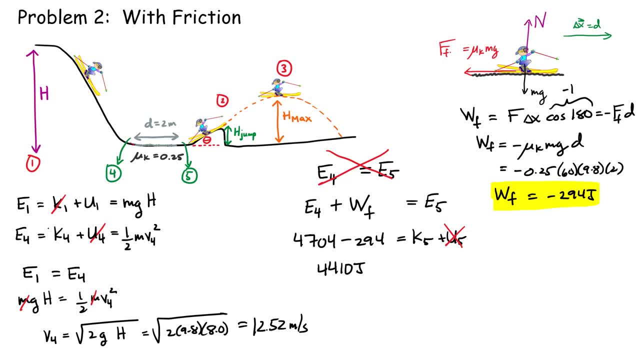 4,410 joules. That's the kinetic energy over here at 0.5.. Well, let me just kind of get rid of the unit here. Just call that K5.. Well, let's put it back. Okay. So once you know the kinetic energy, 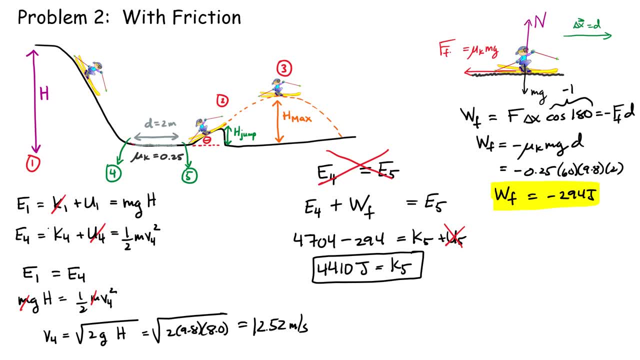 at 0.5,. you can also tell me how fast it's moving over here, right? Because once you know kinetic energy at any point, you automatically know the speed. Okay, So the speed at 0.5,. still on the. 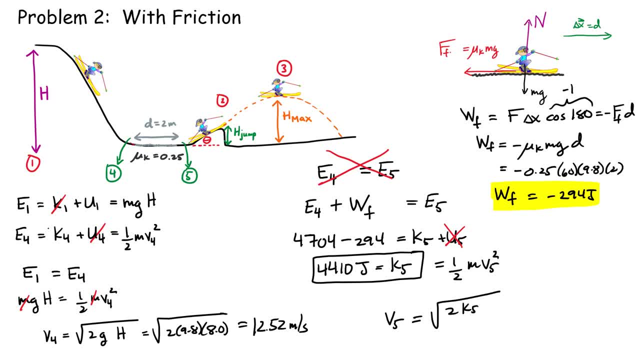 flat section simply 2K5 over the mass. Again, we put our numbers in the calculator and here you should get 12.12 meters per second. So you've slowed down a little bit, right? You started off at 12.52 and now you're at 12.12.. So that kind of physically makes sense. right, You've slowed. 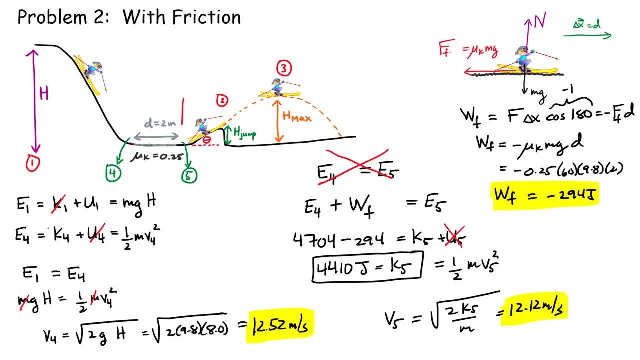 down a little bit here, All right. Now, once you're past this point, again, we are going to have conservation of energy. So the problem is going to be the same thing as the first part, except instead of using this value, guess what You're simply going to use. 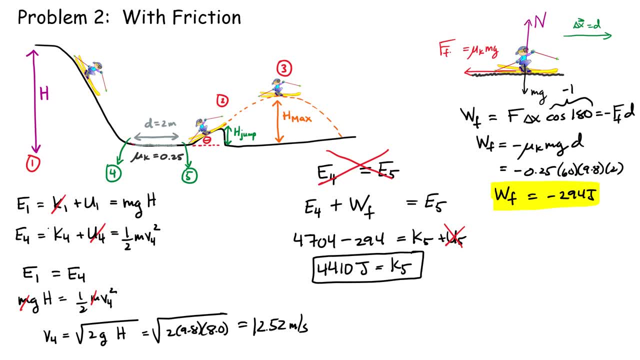 back. okay, so once you know the kinetic energy at 0.5, i can, you can also tell me how fast it's moving over here, right, because once you know kinetic energy at any point you automatically know the speed. okay, so the speed at 0.5, still on the flat section, simply 2 k5 over the mass. again we put 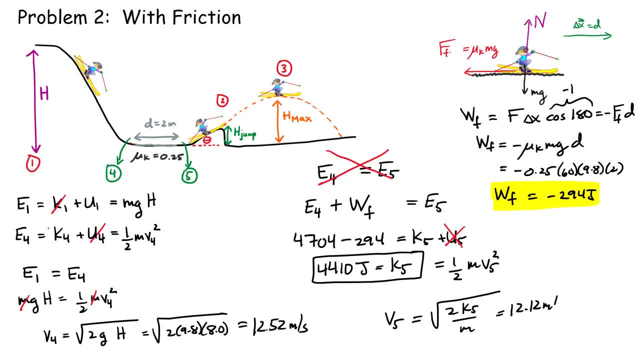 our numbers in the calculator, and here you should get 12.12 meters per second. so you've slowed down a little bit, right, you started off at 12.52 and now you're 12.12, so that kind of physically makes sense. right, you've slowed down a little bit here. 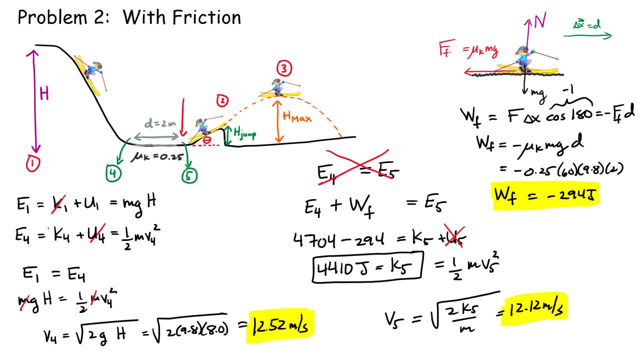 all right. now, once you're past this point, again, we are going to have conservation of energy. so the problem is going to be the same thing as the first part, except, instead of using this value- guess what? you're simply going to use this value, right? because from 0.5 to 0.2 we have 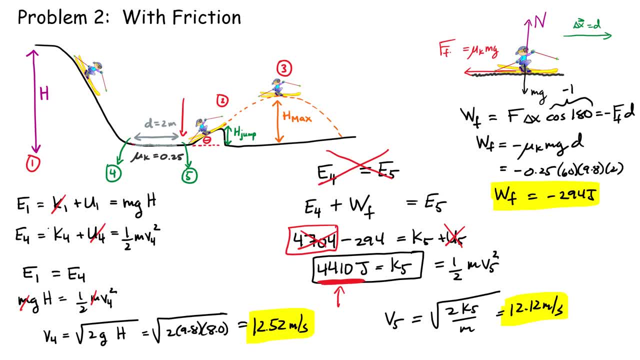 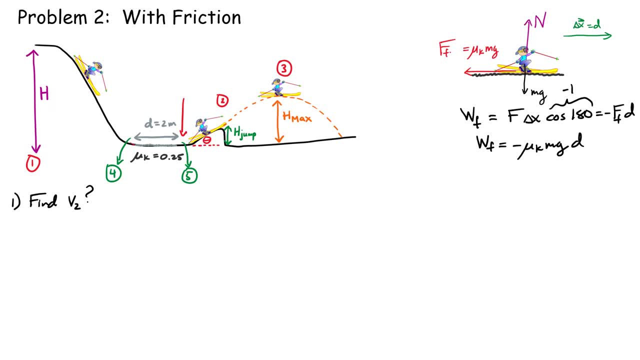 conservation of energy, and from 0.2 to 0.3 we have conservation of energy. yeah, so to find v2, then that's the speed here at the top of the jump. all you have to do is set these equal to each other, right? so you have the energy at 0.5 again. that's all. 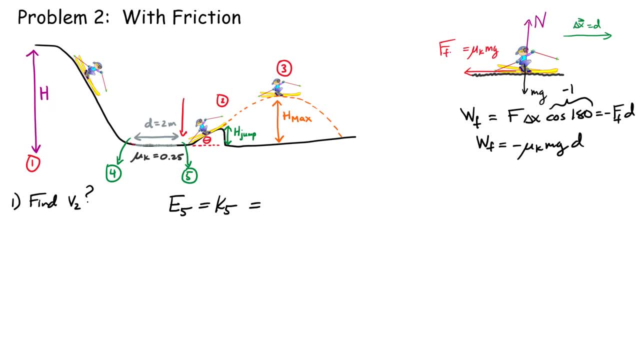 kinetic energy at 0.5. this here has to be equal to the total energy at 0.2. that's one half mv2 squared plus mg and the height of the jump. again, that's the potential energy at the top, and this guy you can automatically calculate right, that's an easy number to get. actually, this guy here i had. 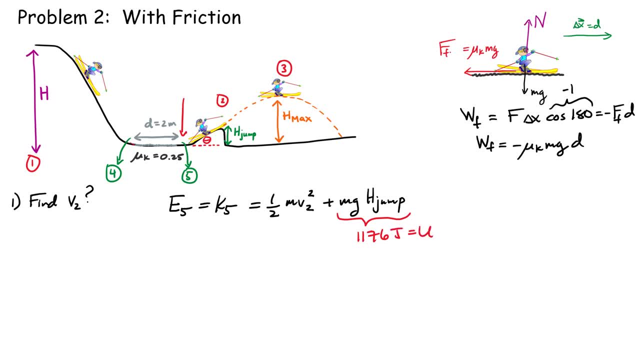 76 joules. right, that's the potential energy here, um at 0.2. so, uh, putting the numbers here now, kinetic energy at 0.5, we said, was 44, 10 equals to one half mv2 squared, and then plus 11, 76. 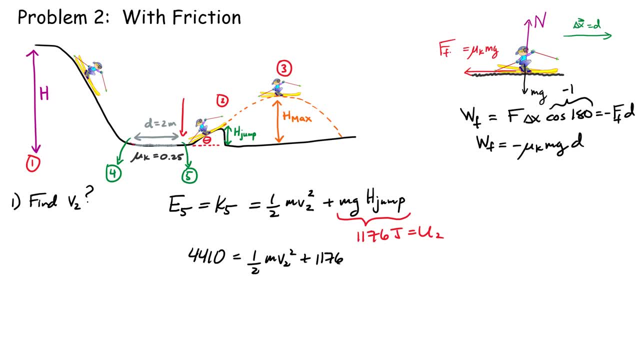 all right, all you have to do is just substitute the mass and do a little bit of algebra. you should get that v2 is equal to the square root of this, so 244- 10 if i do the algebra correctly and divide it by 60.. okay, you put that in the calculator. i get 10.38. 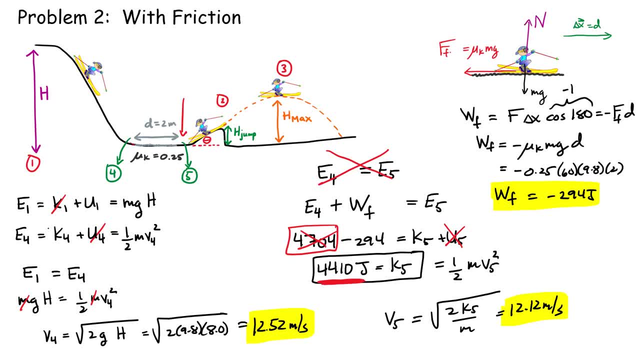 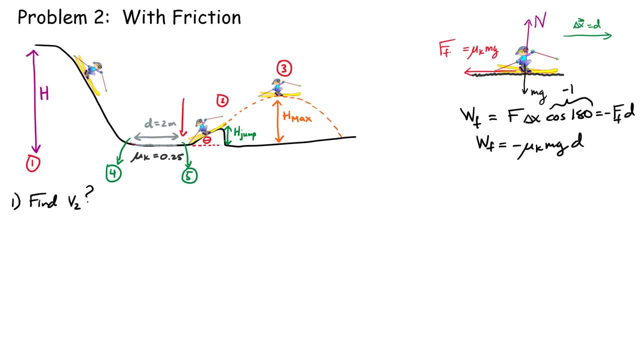 this value? right, Because from 0.5 to 0.2, we have conservation of energy, And from 0.2 to 0.3, we have conservation of energy. Yeah, So to find V2, then that's the speed here at the top of the. 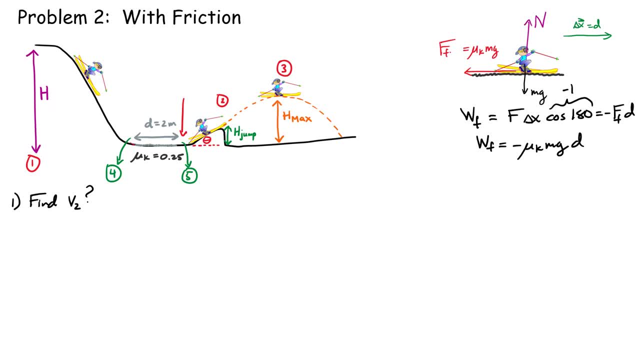 jump. All you have to do is set these equal to each other, right? So you have the energy at 0.5.. Again, that's all kinetic energy at 0.5.. This here has to be equal to the total energy at. 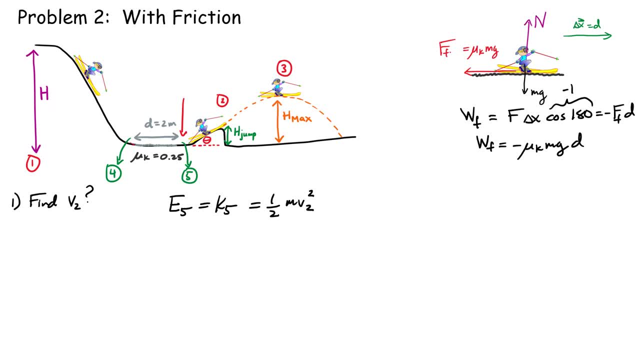 0.2.. That's one half MV2 squared plus MG and the height of the jump. Again, that's the potential energy at the top. And this guy you can automatically calculate, right, That's an easy number to get. Actually, this guy here I had 1176 joules right. That's the potential energy. 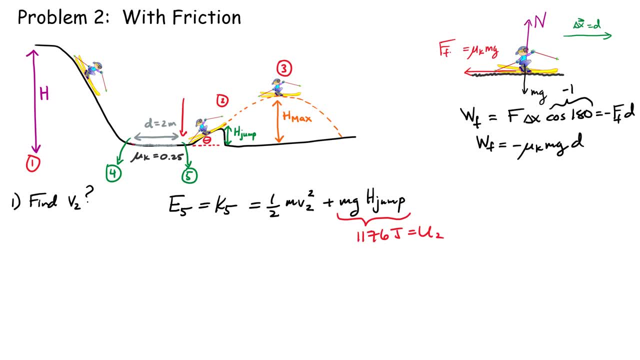 at 0.2.. So putting the numbers here now, kinetic energy at 0.5, we said, was 4410, equals to one half MV2 squared, and then plus 1176.. All right, All you have to do is just. 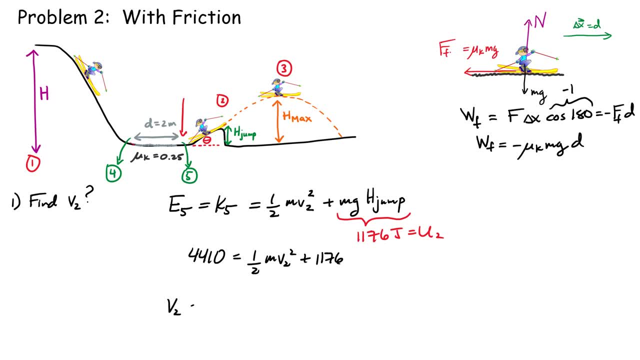 substitute the mass and do a little bit of algebra, You should get that V2 is equal to the square root of this, So 24410, if I do the algebra correctly, divided by 60.. Okay, You put that in the calculator. I get 10.38 meters per second. 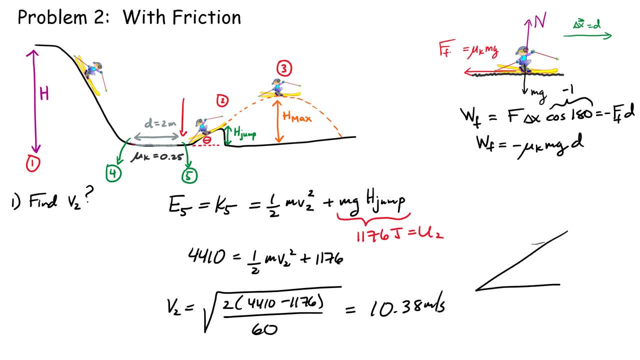 Now again, remember, this is at the top of the ramp, So I'm launching here at an angle of 45 degrees, just like I did before, except now my speed is 10.38 meters per second, And this angle here is 45 degrees. So now we proceed using the exact same approach as before. 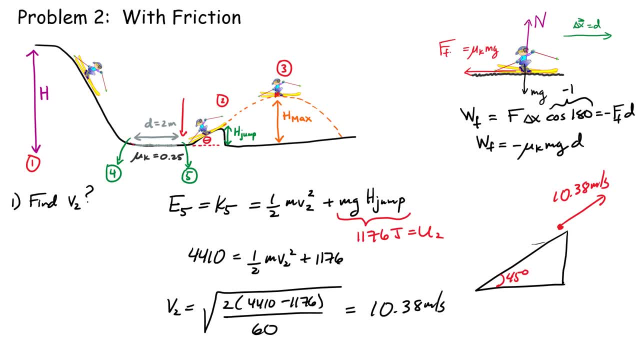 What I'm interested in now is at the top And at the top we know that V2, Vy is equal to zero, but we know that Vx is the same everywhere throughout this projectile motion part of the problem, right. So Vx here has to be, this has to be V. 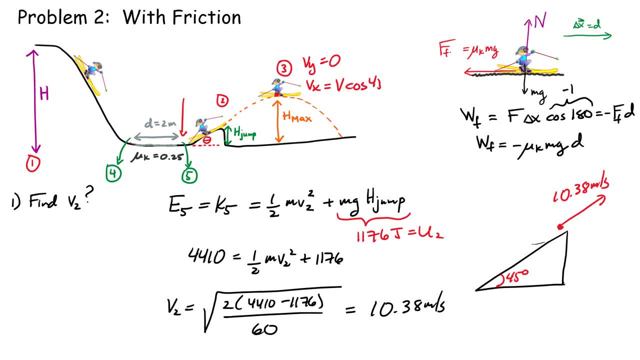 cosine of 45 degrees. Let's try that again, All right. So let's go ahead now and write down our expression equating the energy at 0.2 to 0.3, and then solving for the maximum height in this case. All right. So to introduce Hmax again, we simply use the 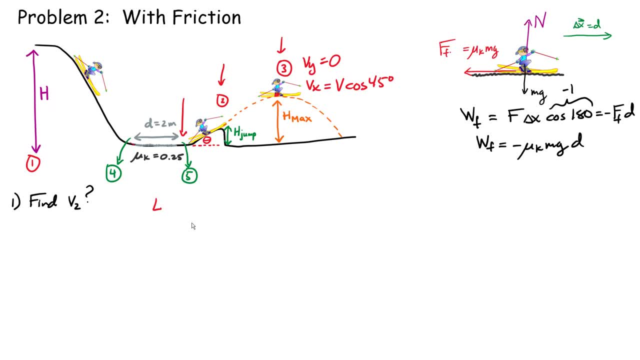 conservation of mechanical energy, and I could do that for 0.5.. Let me just switch the color here. The energy at 0.5,, we know, has to be equal to the energy at 0.2,, has to be equal to the total. 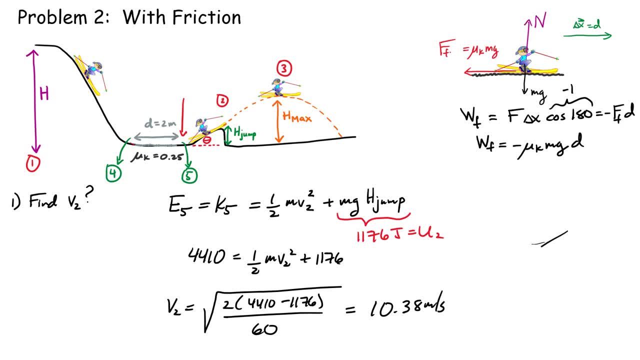 meters per second. now again, remember, this is a at the top of the ramp, so i'm launching here at an angle of 45 degrees, just like i did before, except now my speed is 10.38 meters per second and this angle here is 45 degrees. so now we proceed using the exact same approach as before. 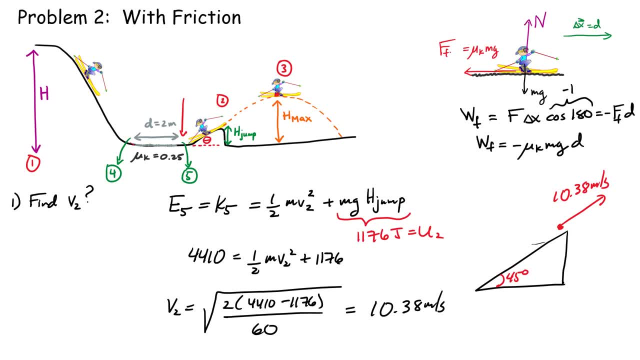 what i'm interested in now is the at the top and at the top. we know that vy is equal to zero, but we know that vx is the same everywhere throughout this projectile motion part of the problem, right? so vx here has to be- this, has to be- v cosine of 45 degrees. let's try that again, all right. so let's go ahead now and write down our 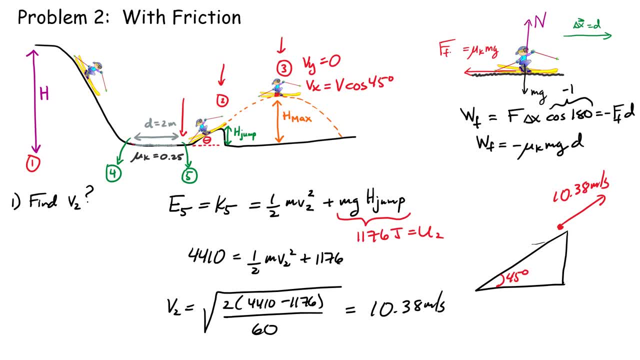 expression equating the energy of 0.2 to 0.3 and then solving for the maximum height in this case. all right. so to introduce h max again, we simply use conservation mechanical energy, and i could do that for 0.5. let me switch the color here. the energy at 0.5, we know, has to be equal to the 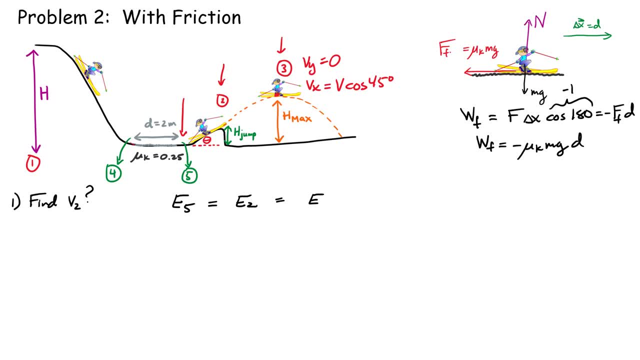 energy at 0.2 has to be equal to the total mechanical energy at 0.3. at 0.5. we said we only had kinetic energy because we're on the ground at the top of the jump. we just solved that. we had kinetic plus some potential energy at the top. 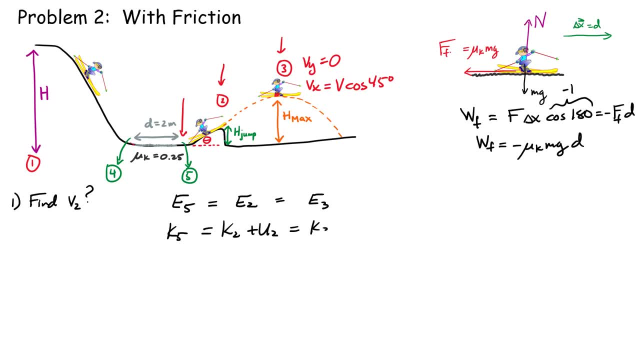 maximum height over here. what we're going to have is some kinetic energy at that top and also some gravitational potential energy at the top. what i'm going to do now, i'm just going to use both of these expressions here, because it's just a little bit simpler. k5- i know, remember k5 was. 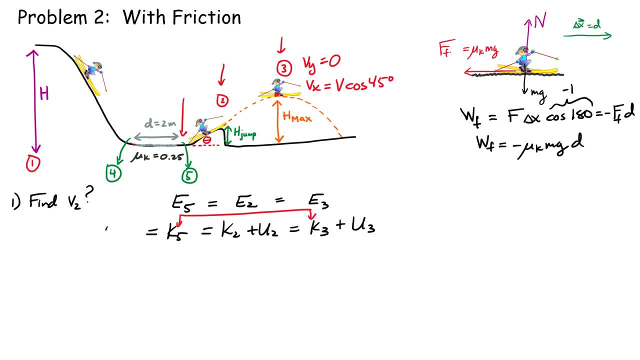 the value. what do we have? 4410, just the number right. that's the number of joules we had after this rough patch. all right now, how do i write this k3 term? well, that's one half m. now it's the speed at the top. at the top, all we have is vx squared. so be careful. 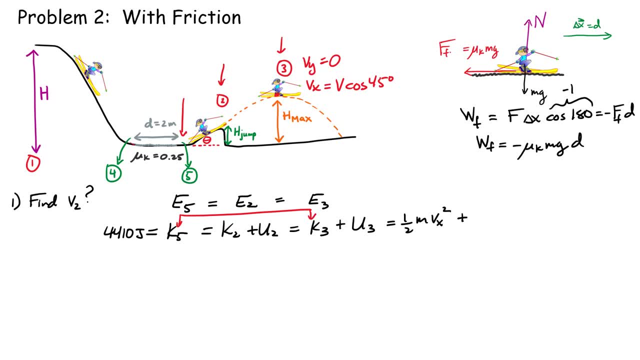 right, it's only that x component that we need, and then, plus how much gravitational potential energy do we have at the top, mg, and that maximum height. this is what we're trying to solve for all right, and all of this here has to be equal to k5. okay, so here's my expression. we have to do some algebra. 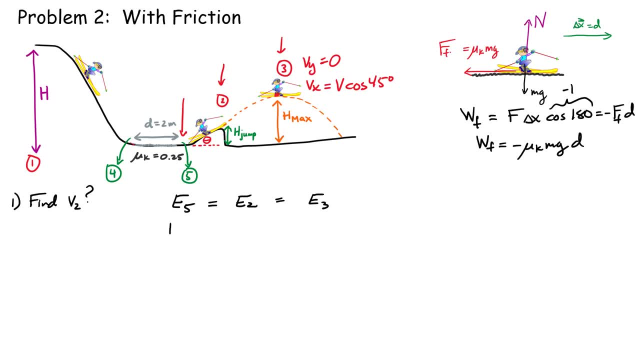 mechanical energy at 0.3.. At 0.5, we said we only had kinetic energy because we're on the ground At the top of the jump. we just solved that. We had kinetic plus some potential energy at the top. 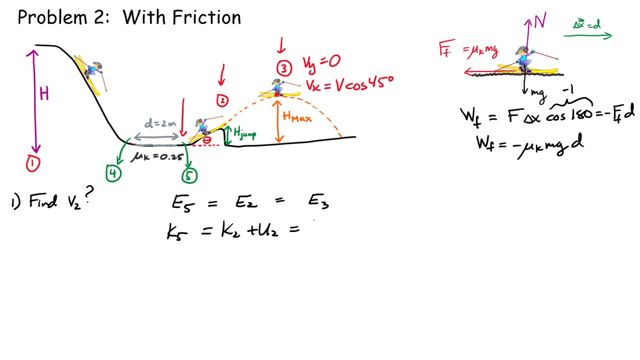 And at the maximum height over here. what we're going to have is some kinetic energy at that top and also some gravitational potential energy at the top. What I'm going to do now, I'm just going to use both of these expressions here, because it's just. 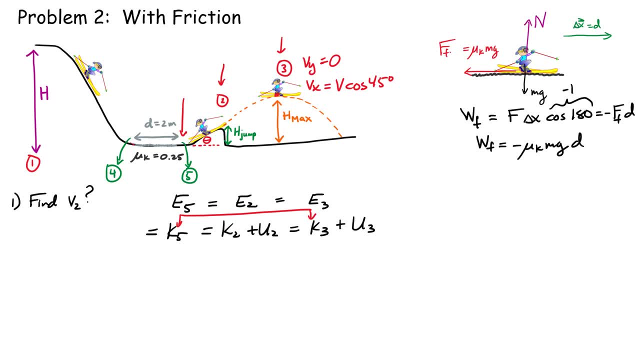 a little bit simpler. K5, I know, Remember, K5 was the value. what do we have? 4,410.. Just the number, right? That's the number of joules we had after this rough patch. All right, Now how do I write this K3 term? Well, that's one half m Now. it's the speed. 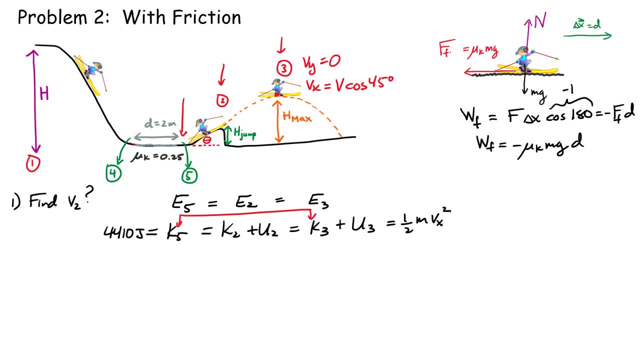 at the top. At the top, all we have is vx squared, So be careful, right, It's only that x component that we need. And then, plus how much gravitational potential energy do we have at the top, mg and that maximum height. This is what we're trying to solve for, All right And all. 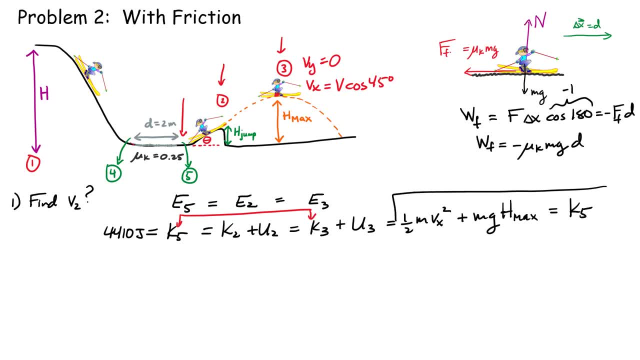 of this here has to be equal to K5.. Okay, So here's my expression. We have to do some algebra now in order to isolate whatever this h max is. So be a little bit careful. You could substitute in some numbers. at this point, I think we're fine. 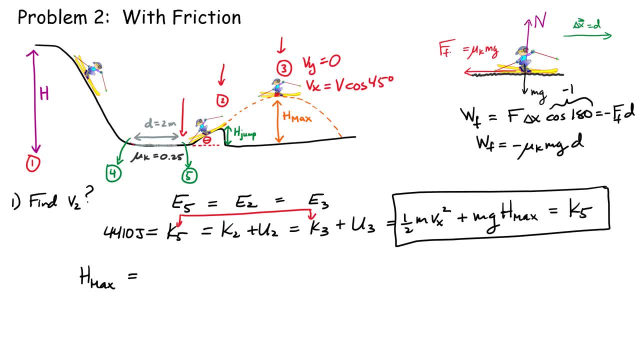 I'm just going to keep on going here. So h max is going to be equal to K5. And I'm going to have to divide through by mg here at the end. Okay, And this other term here, minus one half, If I. 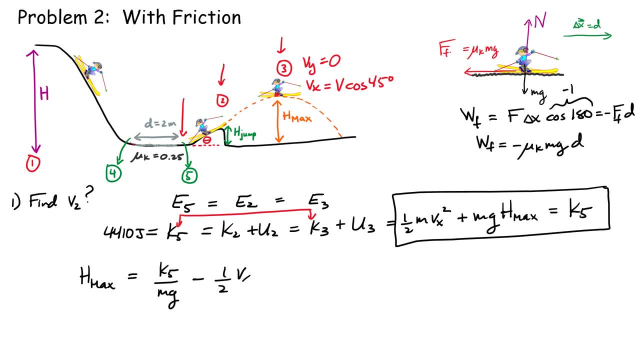 divide through by mg. it's going to cancel out that m And I'm still going to have this guy over little g. All right, Now we substitute our values. All right, So I have 4,410.. The mass was 60.. 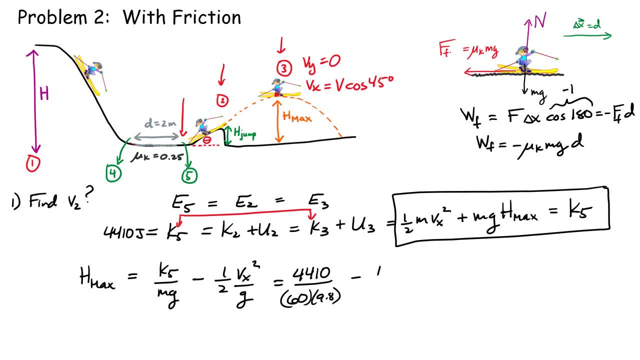 Little g was 9.8.. Okay, Minus one half, Now vx. Now be a little bit careful. Right, It's only the x component, So we have to use this Right, All right. v was 10.38. cosine of 45 degrees. Square that value and divide.